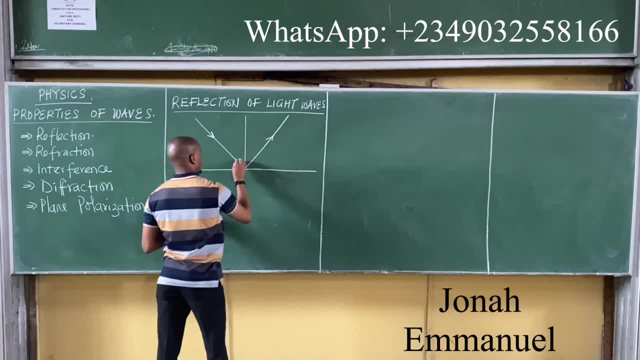 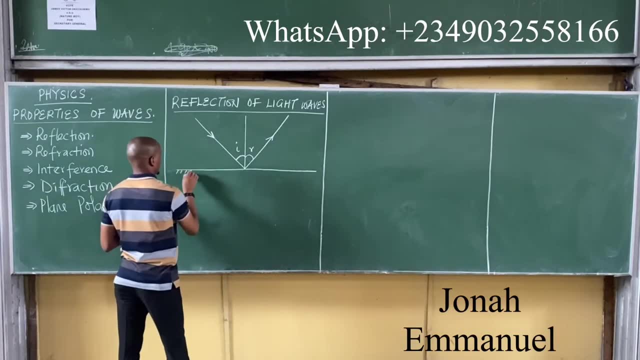 That this is a form of reflection on a visual interface between two media. You can say it's one of these patterns. Is it the same thing? It's a form of reflection, But what does that have to do with the whole idea of reflection? 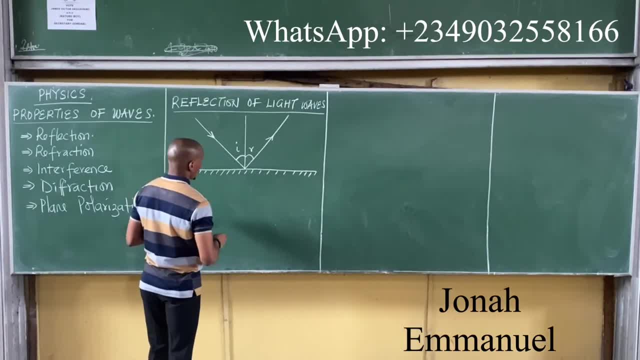 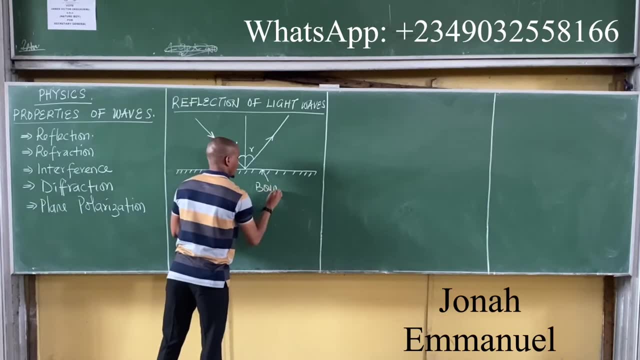 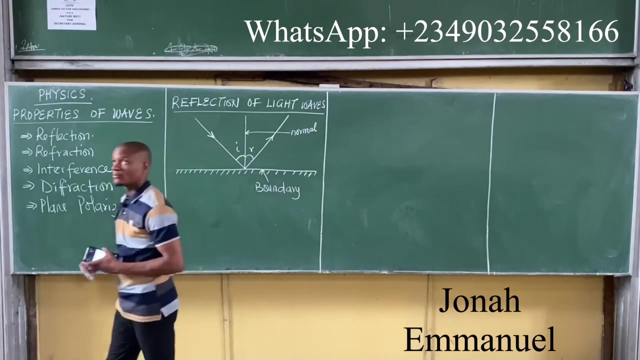 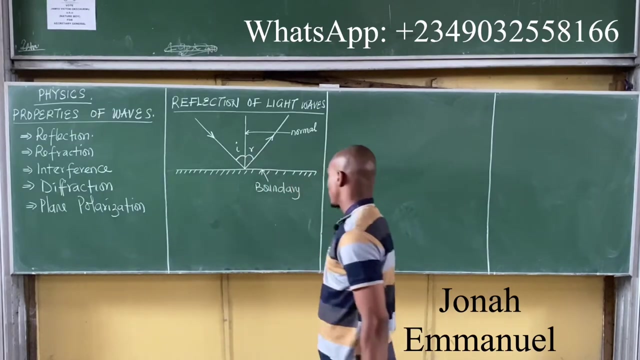 It's a form of representation. What does the third form of reflection look like? So here is the diagram for the flexion right: the flexion part, the diagram here, the flexion part, the diagram here. so what's the flexion? 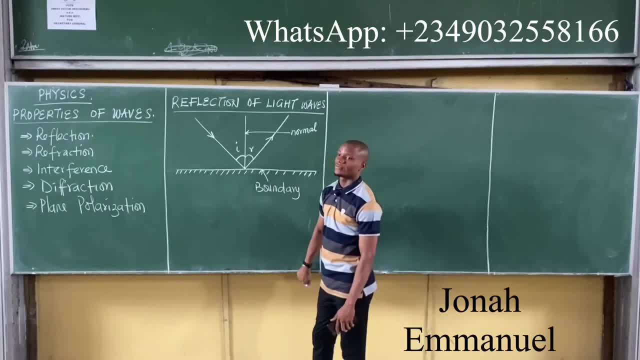 You see what's that? It changes towards the direction of light waves. as it gets to what It bounces, towards the medium. alright, so this light wave is coming this way. so here's the bounce as it hits that one wave. there it goes this way. it has changed direction. 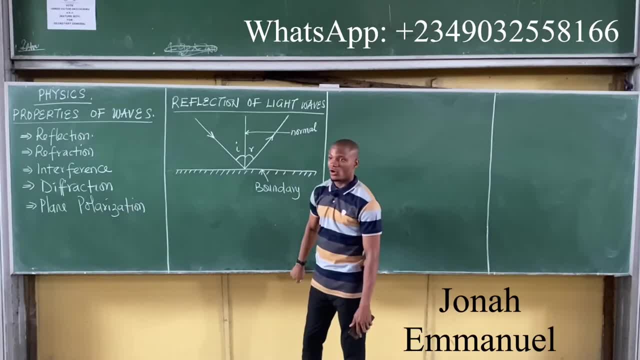 from coming downwards, coming over there upwards, what we call reflection. Now, when it comes to reflection, there's something called AI. there it's called the angle of incidence, some people call it AI, here it's called the angle of reflection. 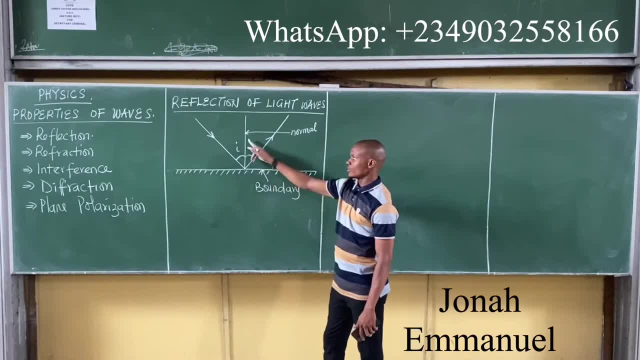 here it's called the boundary, here it's called the normal. What's a normal? Simply a line that makes for a 90 degree width on that line. that's why it's called a normal. So why is it called a normal? 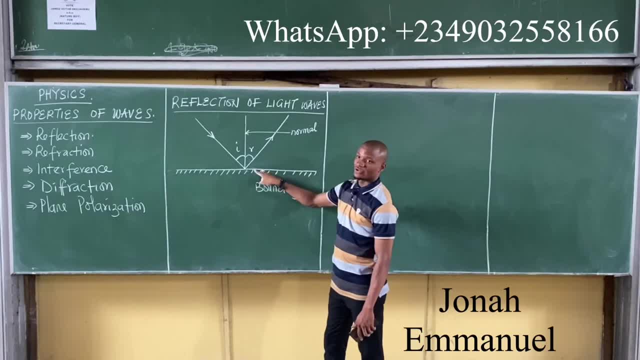 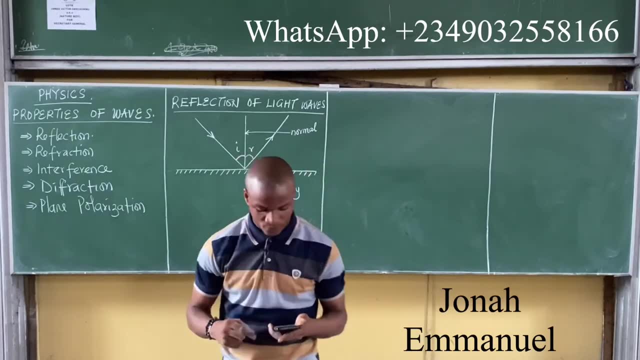 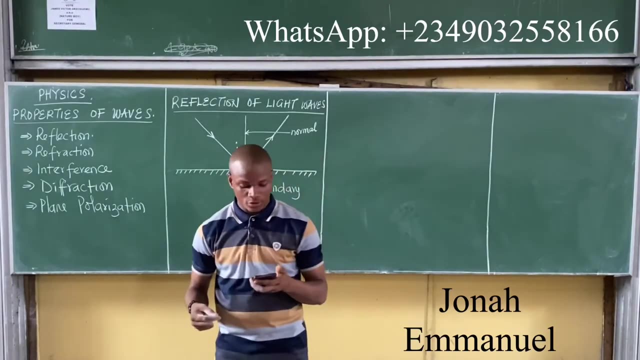 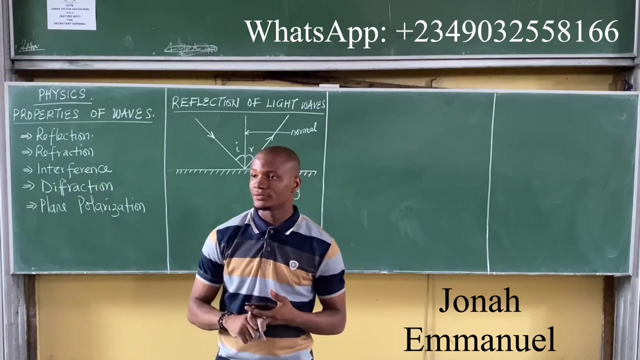 It makes an angle of 90 degree boundary, so it's called the normal to the boundary. alright, but by the way, we'll discuss that in detail shortly. Hold on, please. The angle: the angle which the direction of the motion, the angle which the direction. 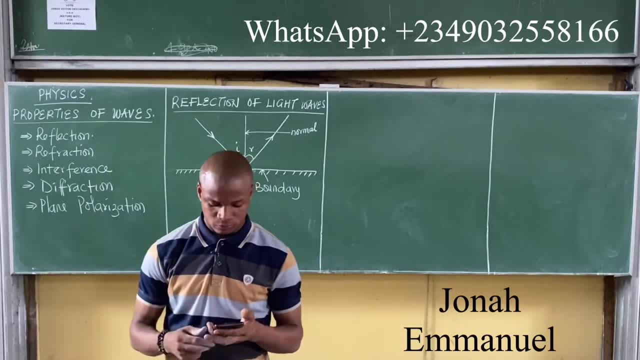 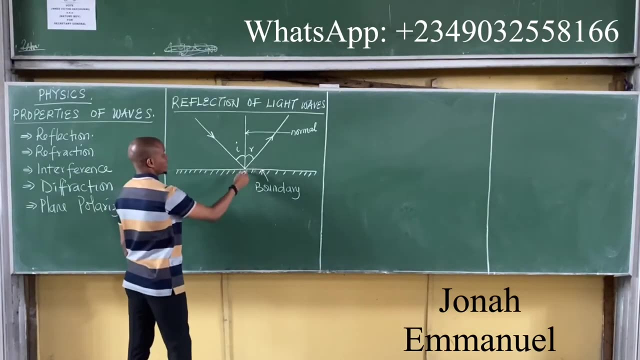 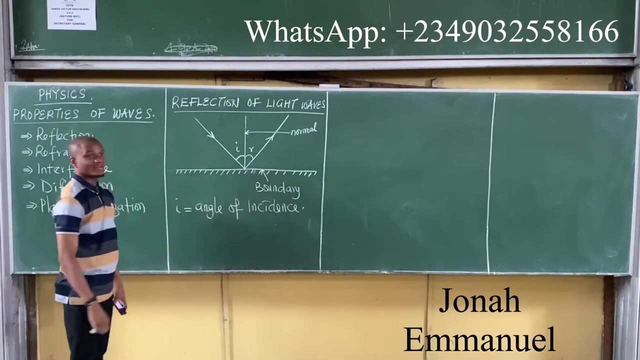 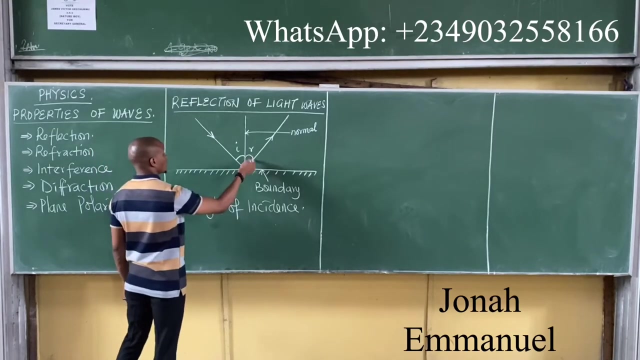 of the motion of the incidence ray, of the incidence ray Mixed with the normal incidence ray. mixed with the normal is called the angle of incidence, so that AI is called angle of incidence and it's called angle of incidence Also also the angle with which the reflected ray. so here's your reflected ray. 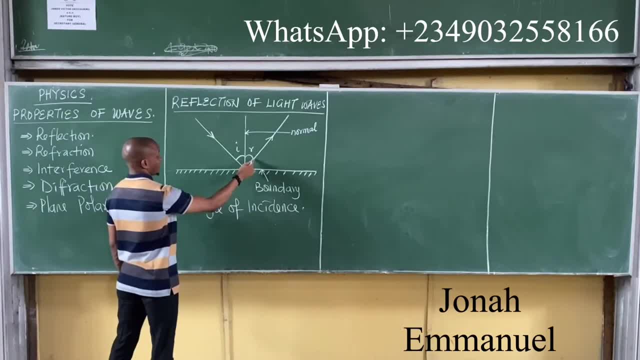 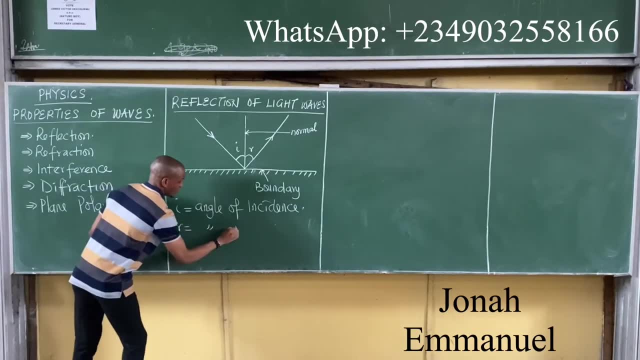 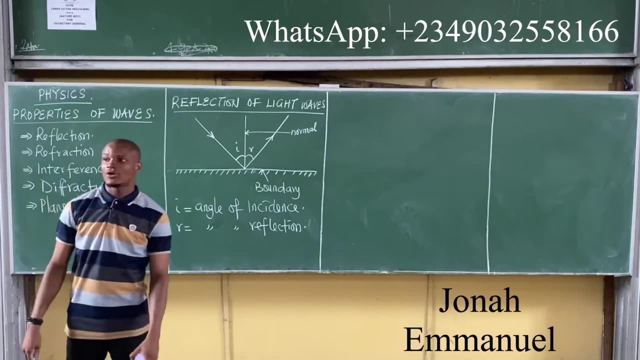 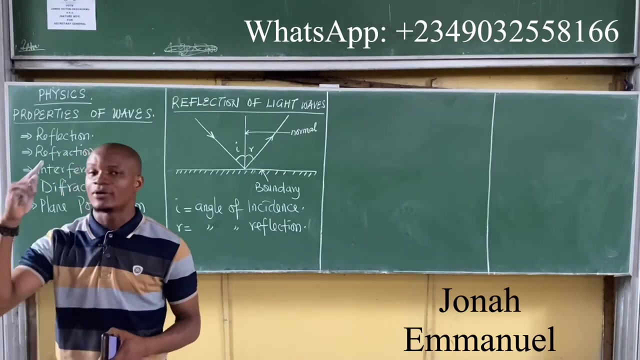 the angle with which the reflected ray mixed with the normal is called the angle of reflection, so AI is called angle of. Why is it called angle of incidence? Why, Because it's the angle between the incidence ray and the normal, R is called angle of reflection. 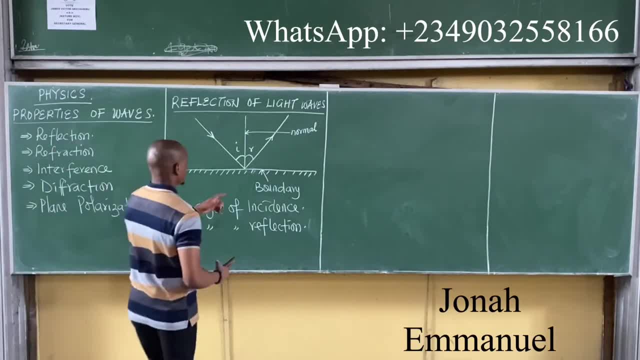 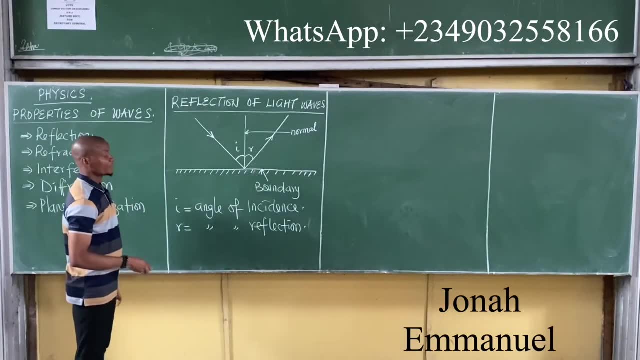 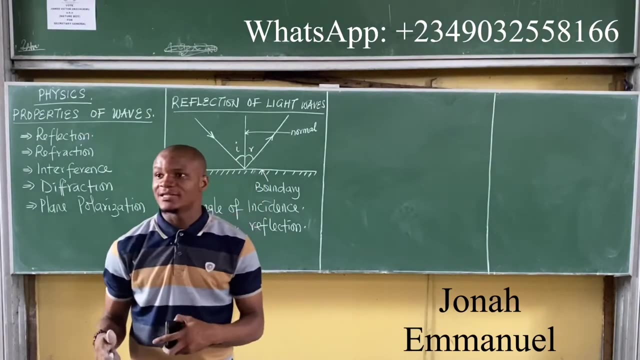 Why? It's the angle between the reflected ray and the normal. This angle here is called angle of reflection. Full stop Paragraph Experiments show that the angle of incidence is equal to the angle of reflection. Okay, So the angle of reflection. 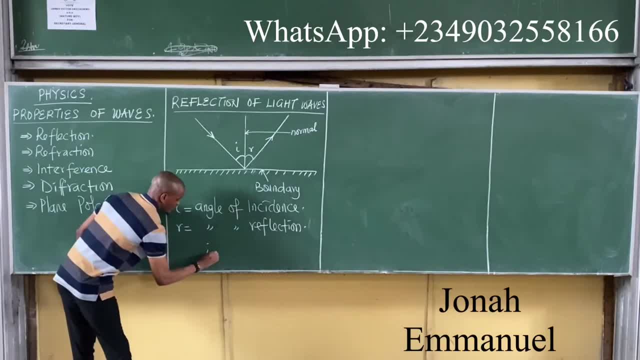 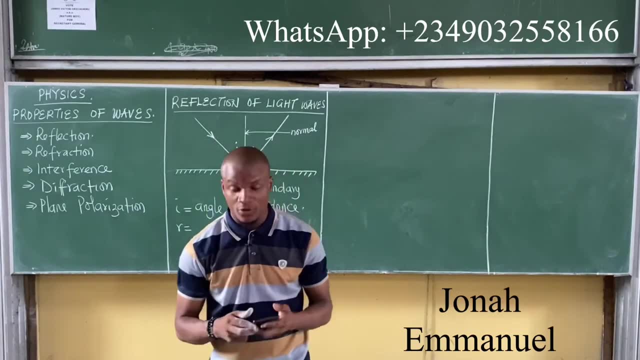 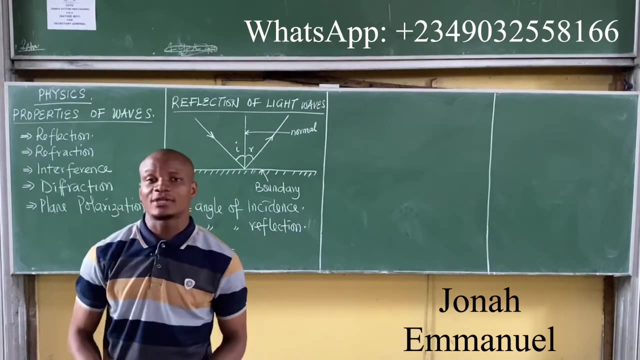 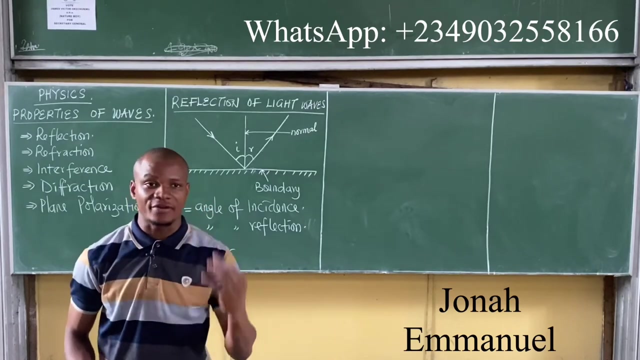 When it comes to reflection, note that I is equal to R, Correct. Correct Shows that the angle of incidence is equal to the angle of reflection. That's for reflection I is equal to R. So question: They tell you. they say light is incident on a glass piece at an angle of 53 degrees. 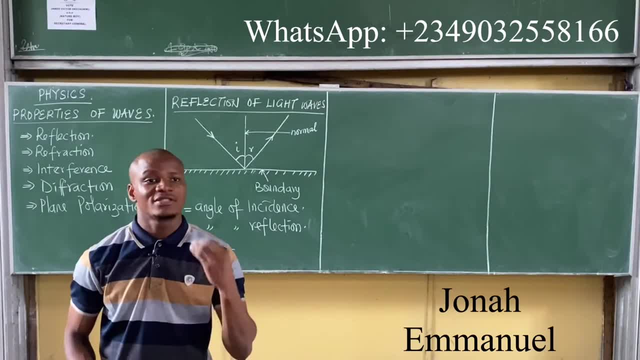 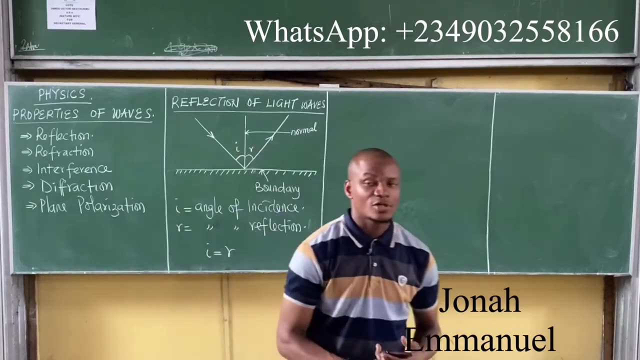 What is the angle of reflection? What's the answer there? Still 53 degrees. Why Angle of incidence is equal to the angle of reflection. That's the first question we will do today. Subheading please. Laws of reflection- Subheading please. 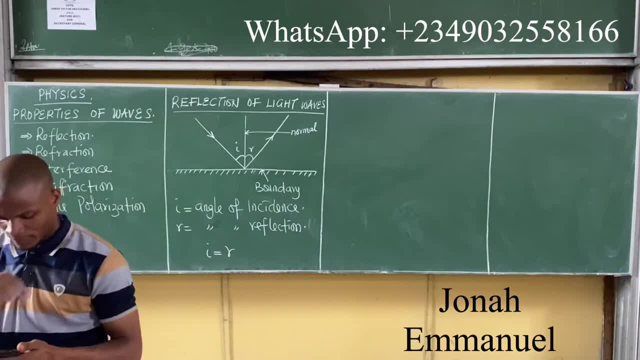 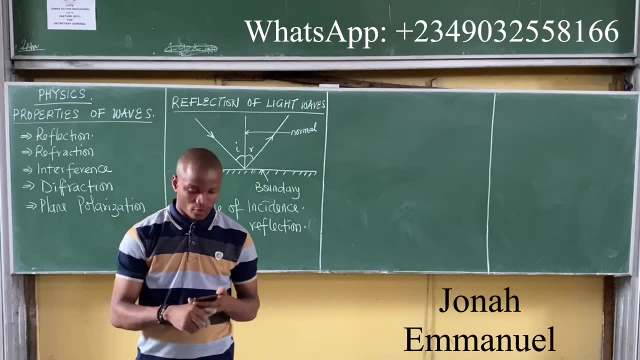 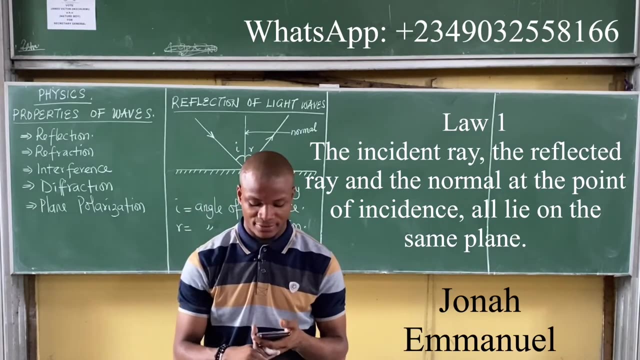 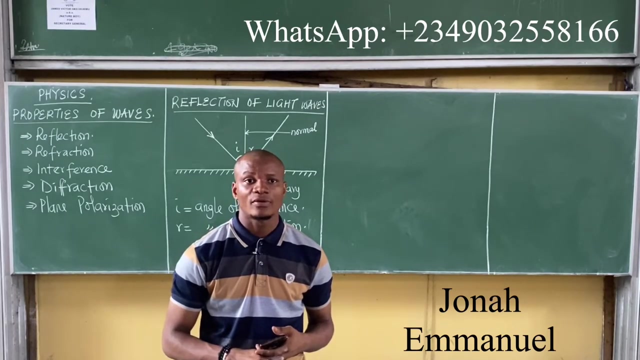 Laws of reflection. Laws of reflection Number one. Number one: The incidence ray, The reflected ray and the number at the point of incidence all lie on the same plane. That's your first law of reflection. Number two: The angle of incidence is equal to the angle of reflection. 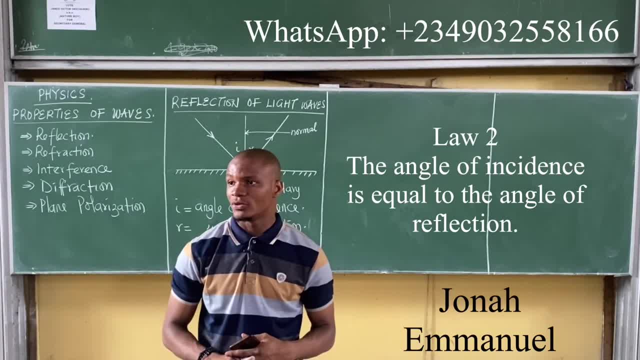 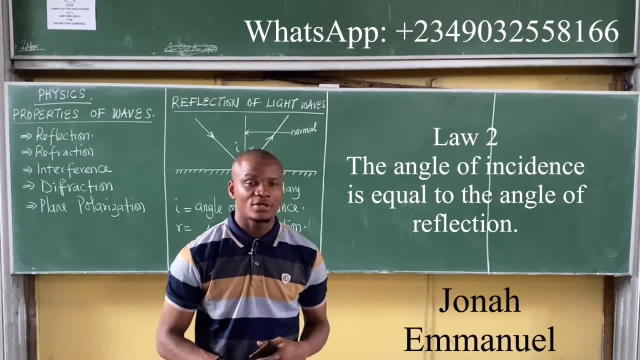 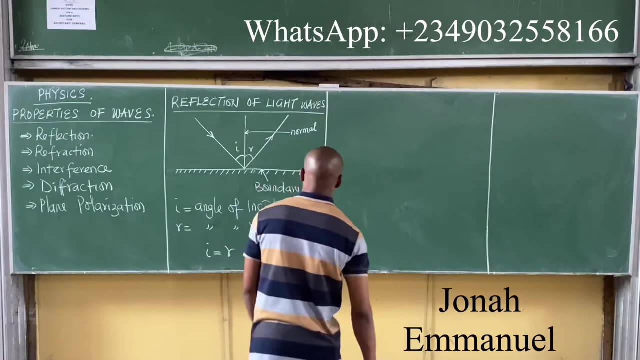 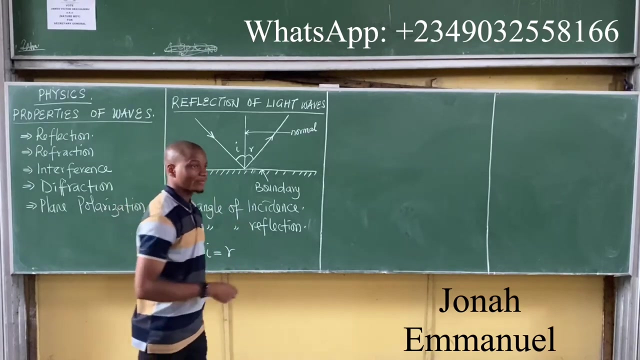 The angle of incidence is equal to the angle of reflection. The angle of incidence is equal to the angle of reflection. Equals to the angle of reflection. Let's do some examples. Let's take a few examples and see what we come up with. 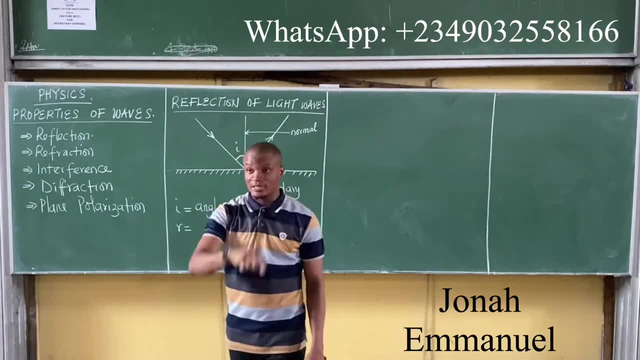 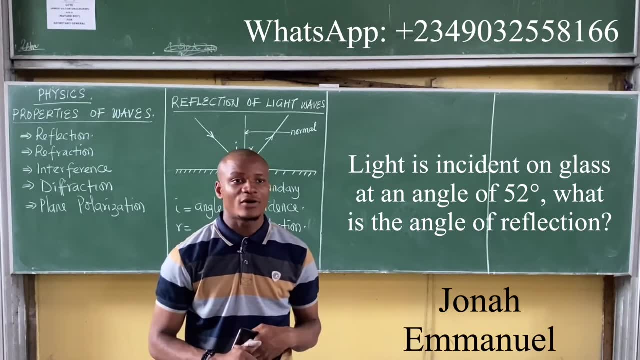 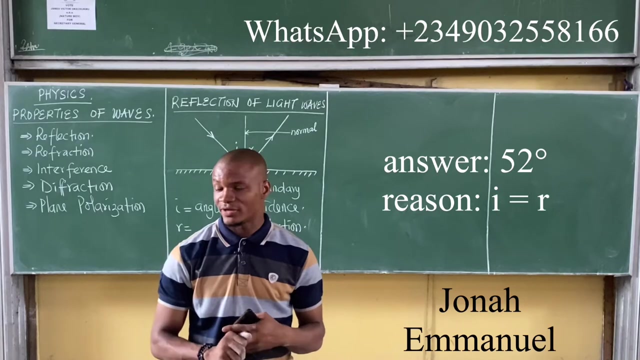 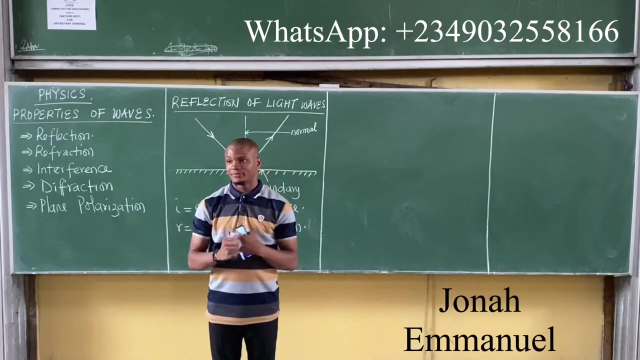 Example one. Example one: light is incident on glass at an angle of 52 degrees. what is the angle of reflection? so put your answer there. what is the angle of reflection? so you put your answer. whatever t right there is correct. okay, example two: just put your answer there. example two: light rays. 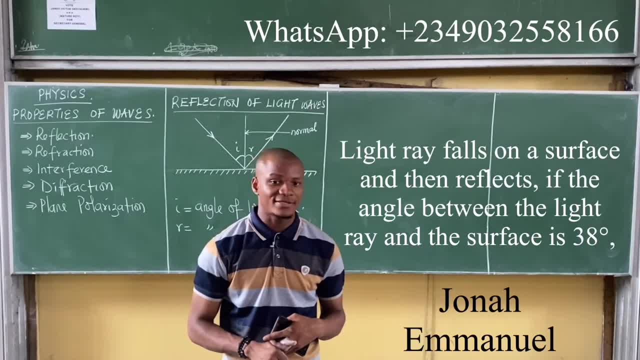 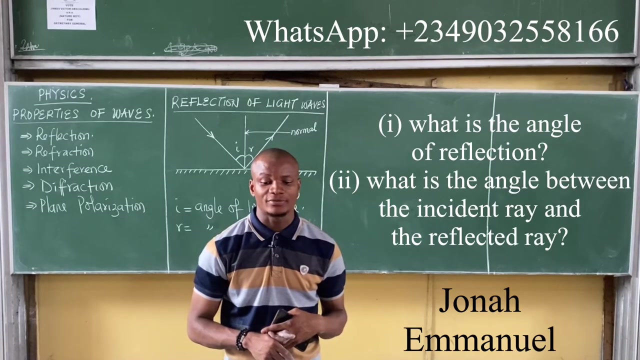 falls on the surface and then reflects. if the angle between the light ray and the surface is 38 degrees and the surface is 38 degrees i, what is the angle of reflection? i i, what is the angle between the incident ray and the reflected ring? all right, so look at this. 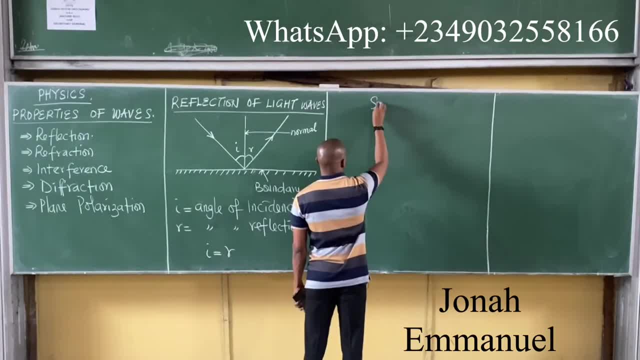 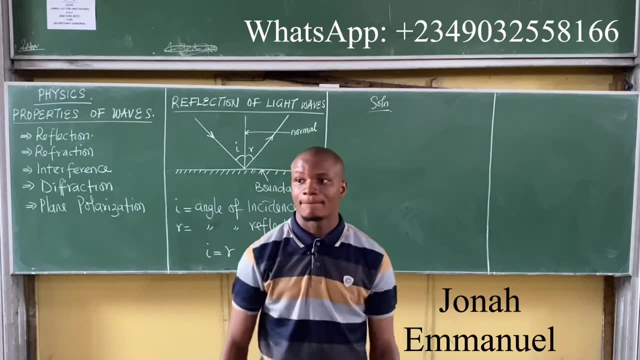 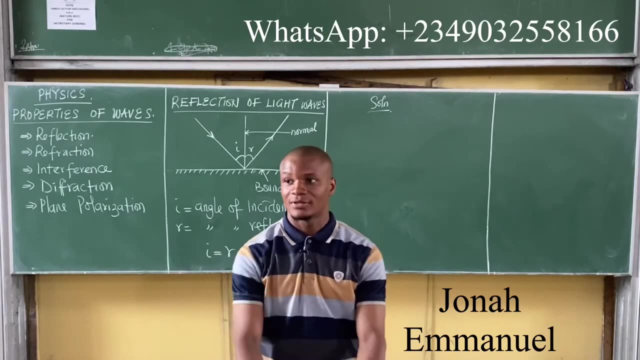 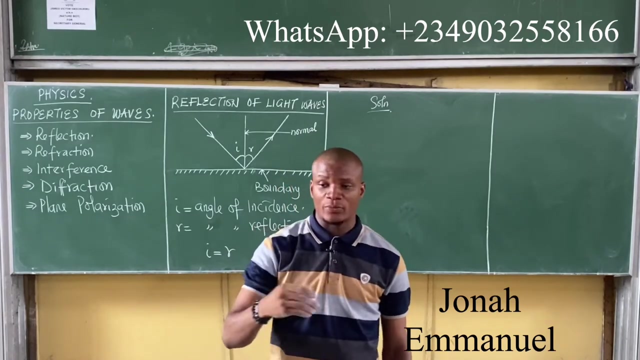 solution. let me ask you, for i, what's the angle of reflection? huh, for i see. what's the angle of reflection? what's our reflection? 38 degrees, that's wrong. so, yes, that's what i want to do. that's why i had to bring out this example. 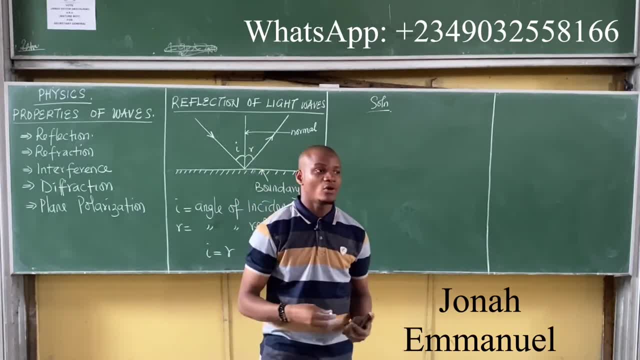 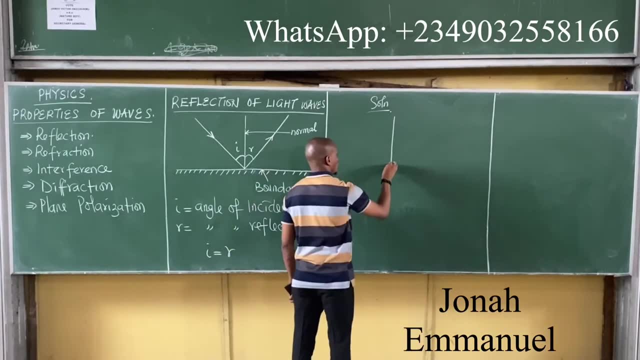 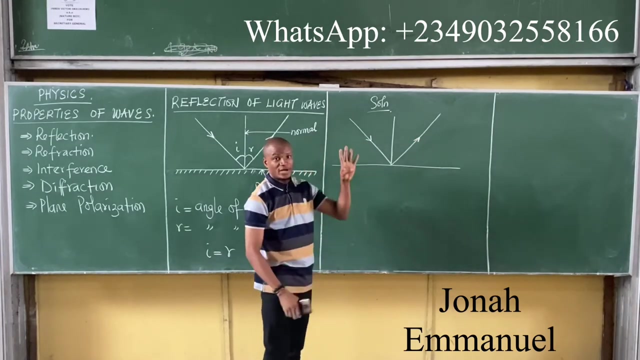 it's not really part of your job, but i think it'll give you a better concept or appreciation of this stuff. look at this now. look at this: when it comes to the concept of reflection, that this is the angle of reflection, there are four possible angles. all right, focus. that's one. here, that's one. 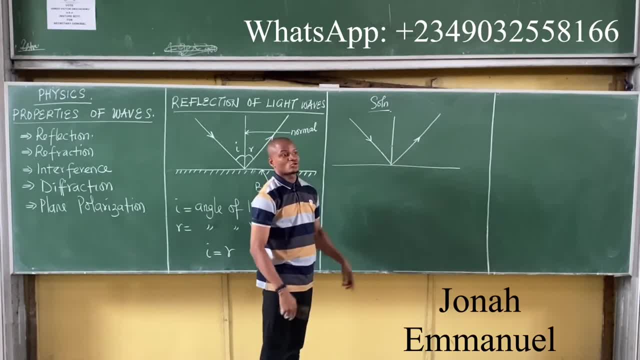 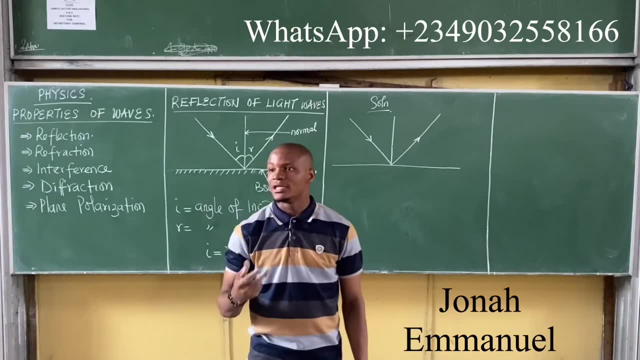 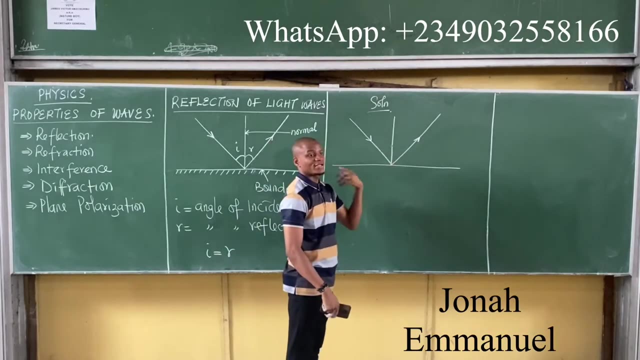 this is two, this is three, this is four. so there are four possible angles there. now, before you answer the question, what's different between the first question and the second one? the first one, you go there, the angle of incidence. that's what this point. what's the angle of incident? we said is: 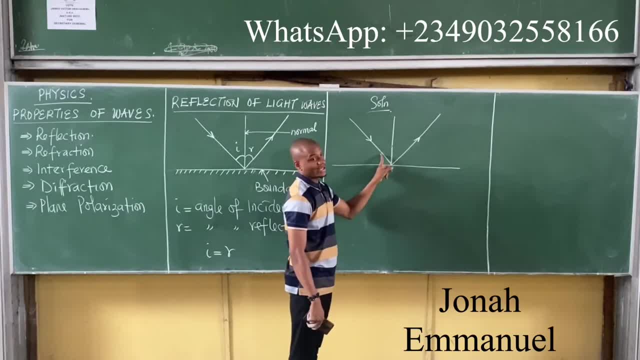 simply the angle between what instead of the number. so if they give you an instant rate for the first question as whatever value of course, from the second law of reflection we say angle of distance is going to go there, angle of reflection. that was the first case in this. 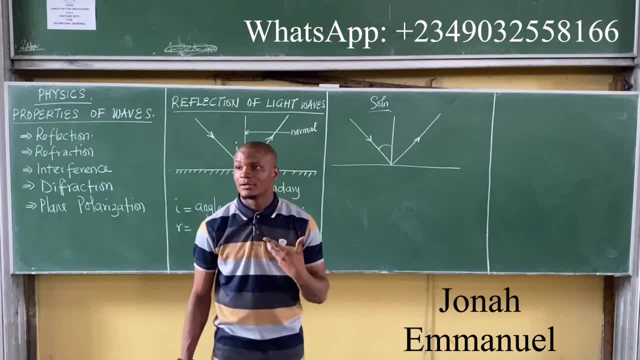 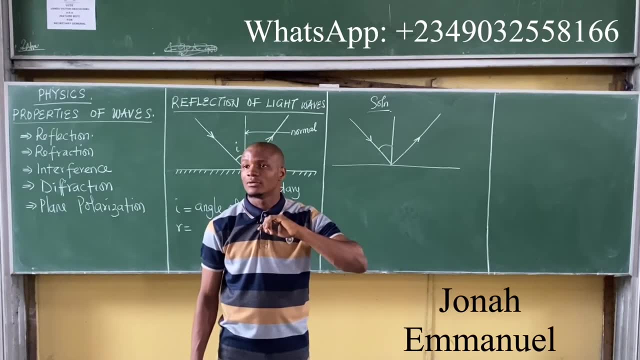 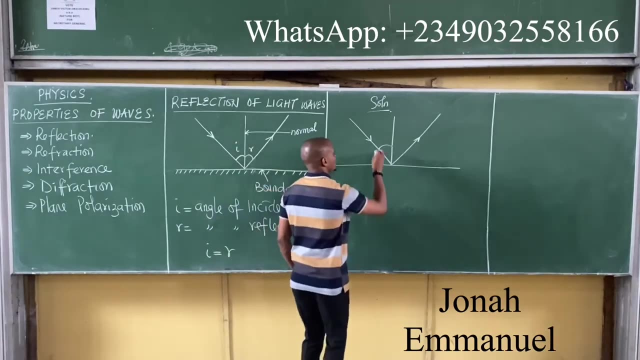 case, i will give you an angle. how many there? 32 degrees, 38 degrees, please check. 38 is between what and what and what is it? the number of the surface? huh, so if i'm looking at, if i call this my um incident rate, we said the angle is 38 degrees. 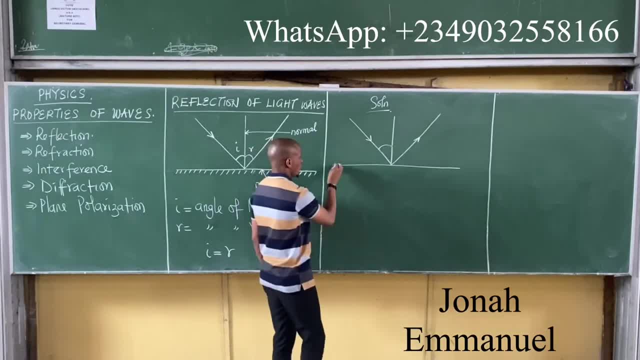 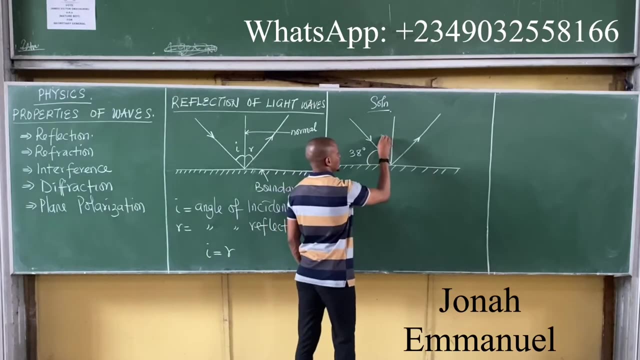 between the instant rate and the surface. where would it be? obviously this is my boundary, or my surface. so when we say 38 degrees, we call this one here, this one here. they gave this as what? 38 degrees. so i'm giving here. this is my eye incident, this is our reflection. 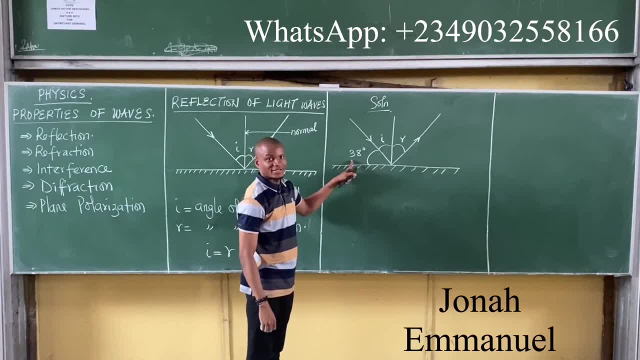 so obviously this is not uh, number of incidents. so what do you hear now? find the value of i. how do you do that? we just say this is called in number. what's it called the number? because this has to get for 90 degrees. so what does it mean? it means that this angle plus this one's equal to over there. 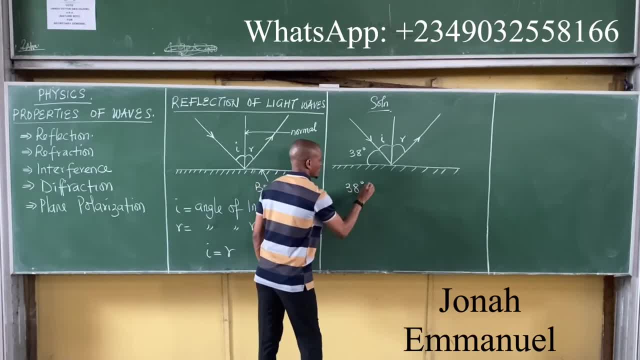 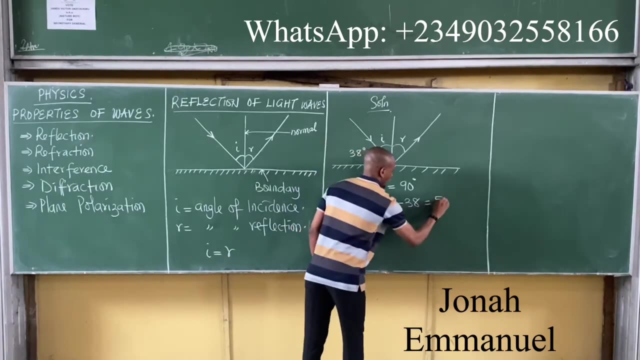 90 degrees, so i have 38 degrees. plus is equal to 90 degrees from here. now, this one was right here, So I have that. my angle of incidence is equal to 90 minus 13.. Do you see what I got there? 52 degrees. 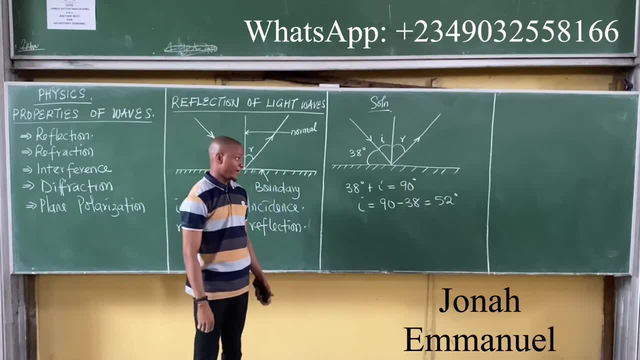 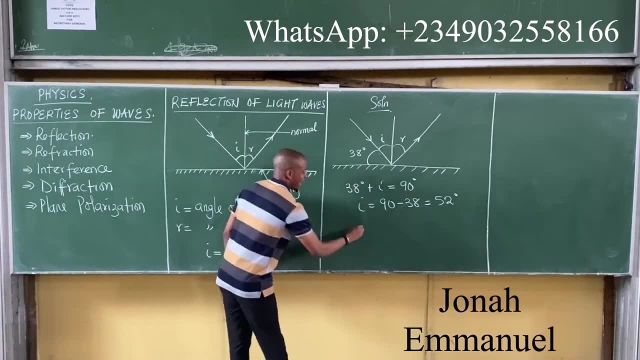 This is the angle of reflection, This is the angle of incidence. And we have to find the angle of reflection. What do we know From second law? we said: I is equal to I. So it means if I get I, automatically I've gotten I. 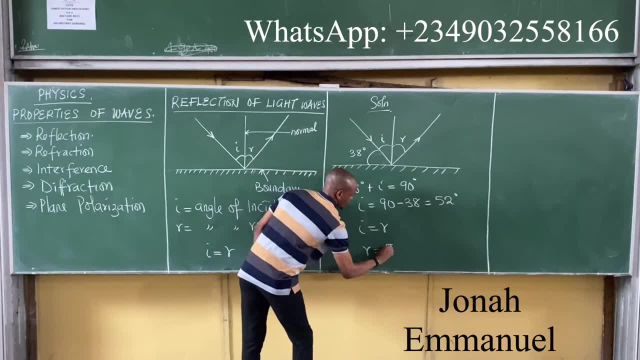 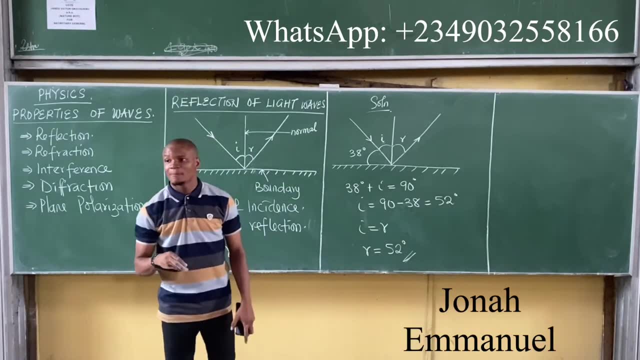 Therefore, the angle of reflection I- you see what I got there- 52 degrees. That's your answer. Now, hold on, That's case one. Case two: what do you got there? What is the angle between incidence rate and reflected rate? 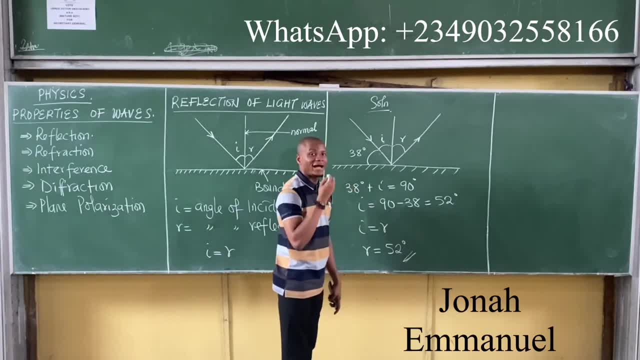 All right, speak of it. So the angle between incidence rate and reflected rate: Where's the incidence rate This point there, Where's the reflected rate, This point there? If I'm taking angle between them, that means the angle between these two. 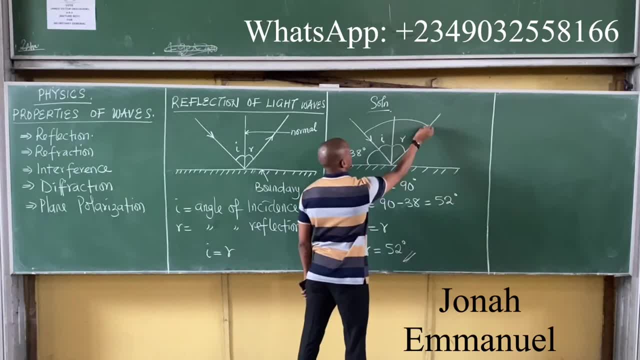 This one and this one. Obviously, it's this angle. So how do I get the angle of this angle Simple, Calculate from here to here plus from here to here. So number two, The angle between the incidence rate and reflected rate. 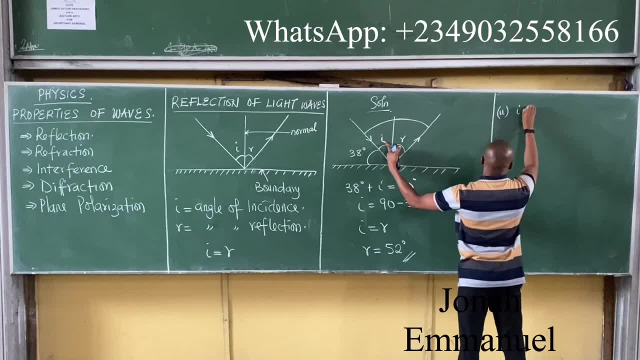 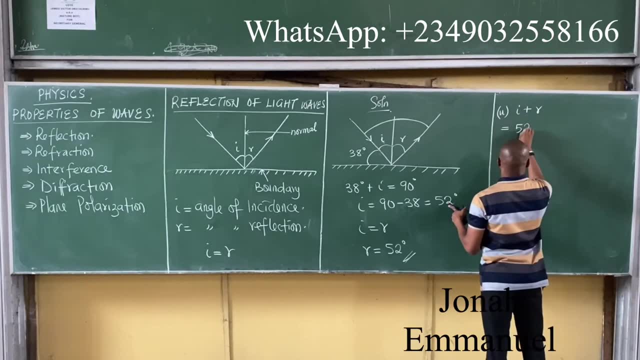 This whole angle becomes my angle of incidence plus my angle of reflection, So it's equal to: this value is 52 degrees plus this value sitting there- 52 degrees, What do you get there? 104 degrees Next, let's do that. 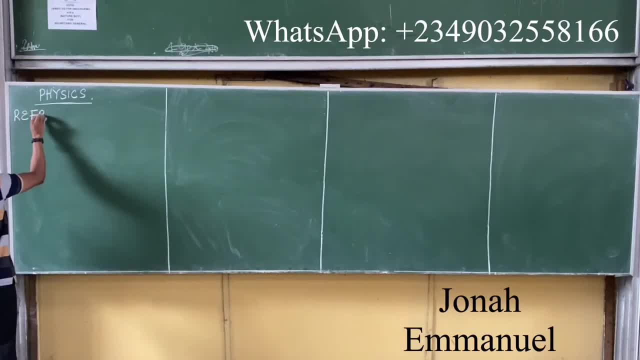 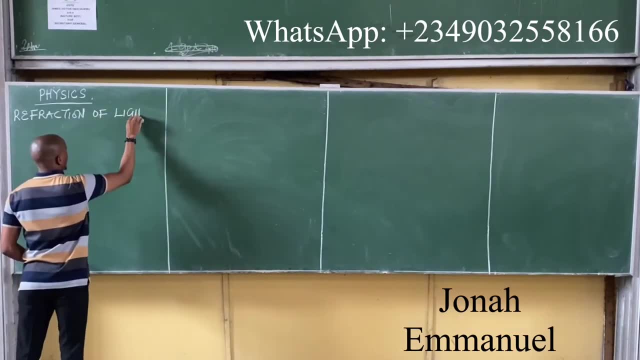 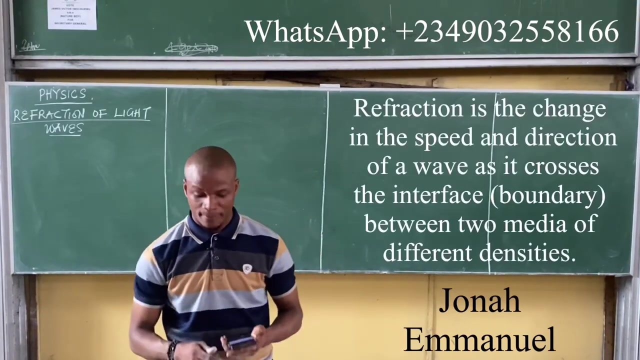 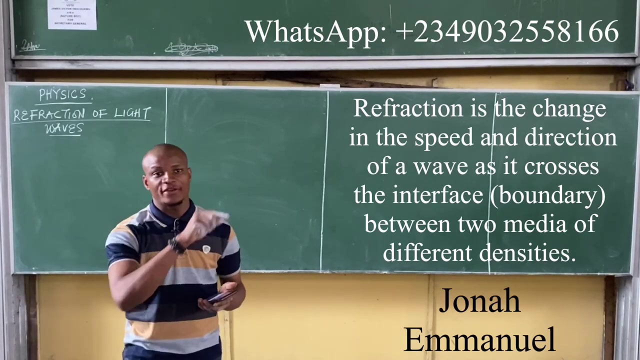 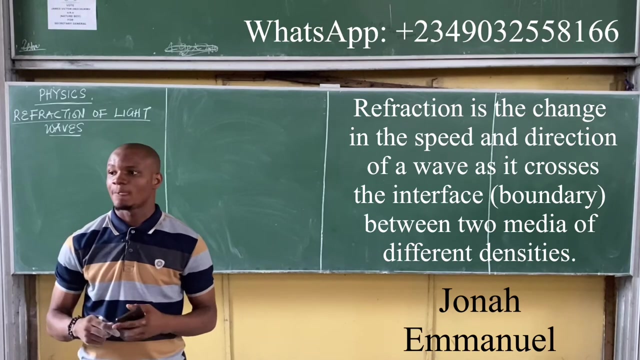 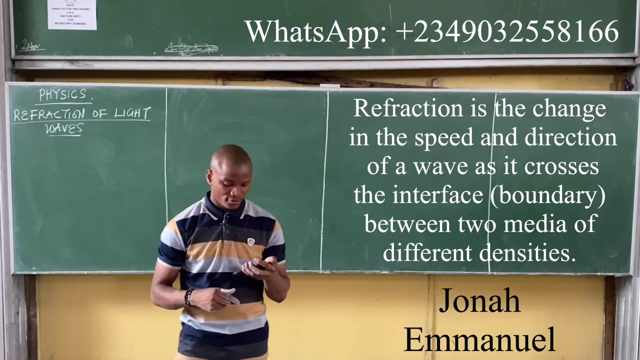 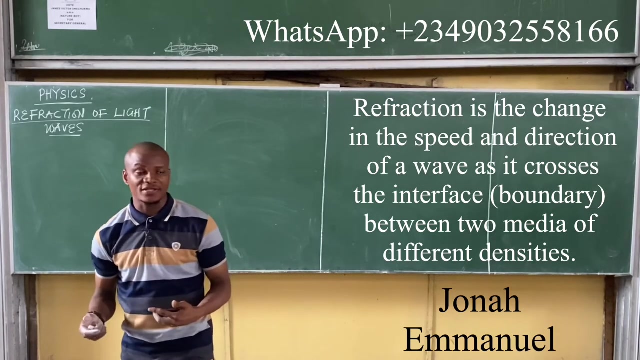 Refraction of light waves. Refraction of light waves- Light waves Definition. Refraction is the change in the speed and direction of a wave as it crosses the interface slash boundary. As it crosses the interface slash boundary between two media, Between two media of different density. 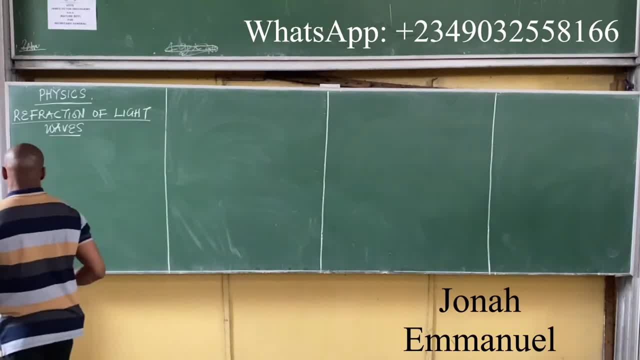 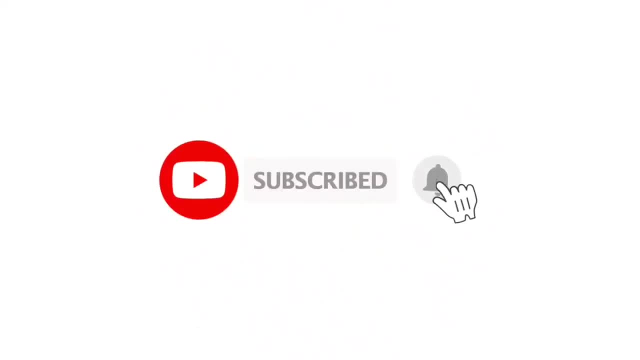 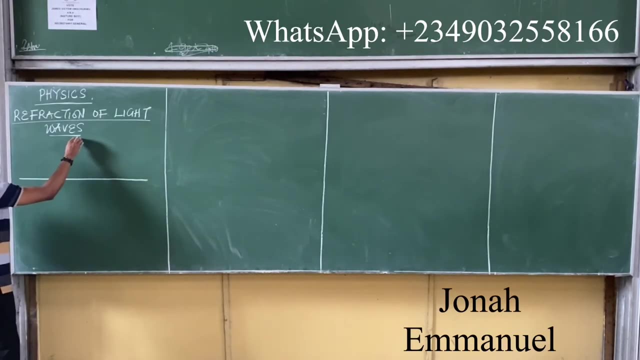 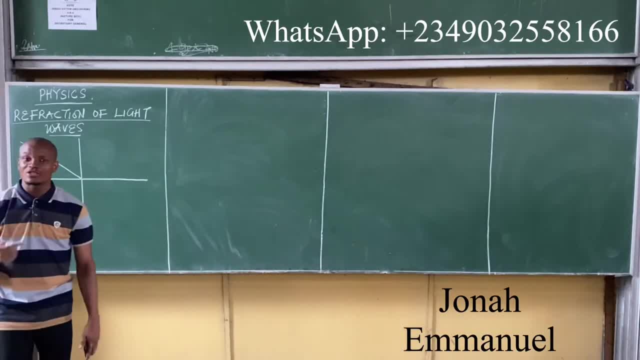 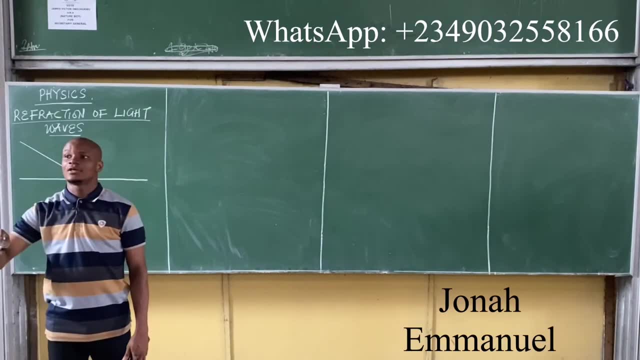 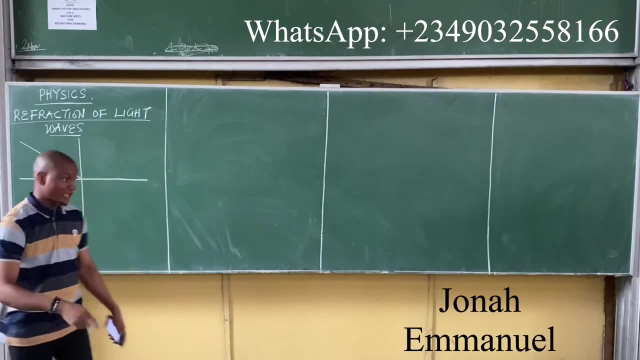 for reflection. the reflected ray does not cut across the boundary right. it comes from a particular medium, hits the boundary and goes back to that same medium. for refraction, it cuts across the boundary, all right. so this man comes to this point. he hits here, he doesn't go this. 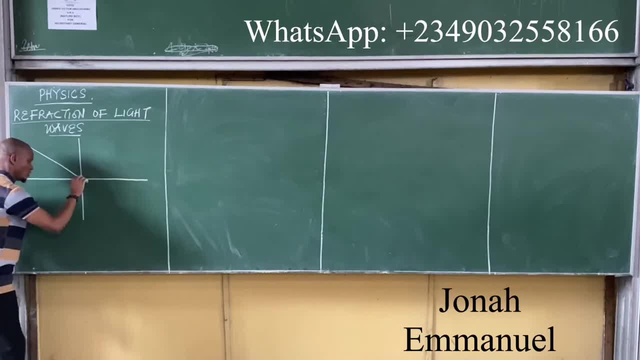 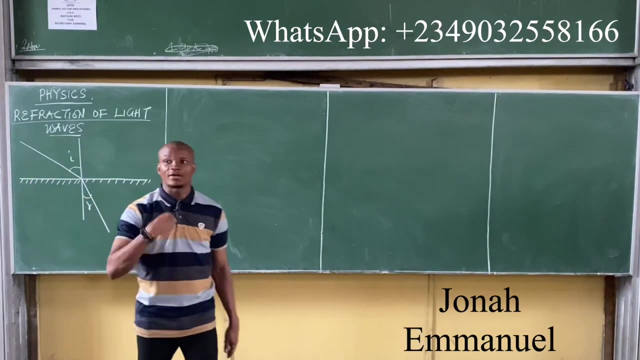 way, he cuts this way and comes down. so it comes this way and it comes out. this is now up. this is now up. to differentiate between reflection and refraction: one of the major differences: that for reflection, the reflected ray goes back to the medium from which it came. for refraction, 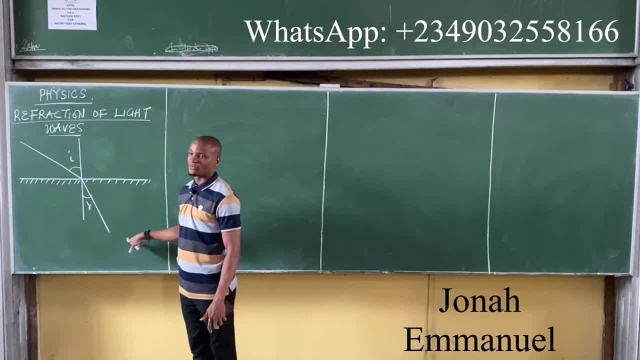 it cuts across that middle and enters a new medium. of course, we said about different densities. all right, that means this medium will have a greater density than this one or a lesser density than the previous, whichever one. so you have this. so this is actually for refraction. think of it. i is called the angle of incidence. 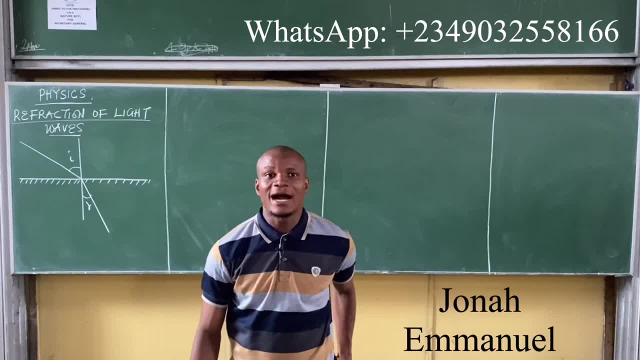 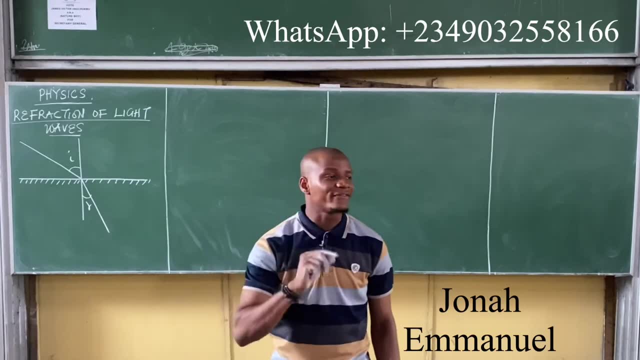 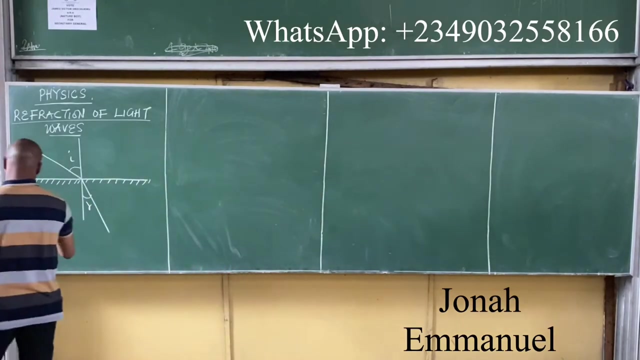 same as the first one there. i is equal to the angle of incidence. yes, y r is equal to the angle of refraction. y r is equal to the angle of refraction. y r is equal to the angle of refraction, so that's right in this case. now i: 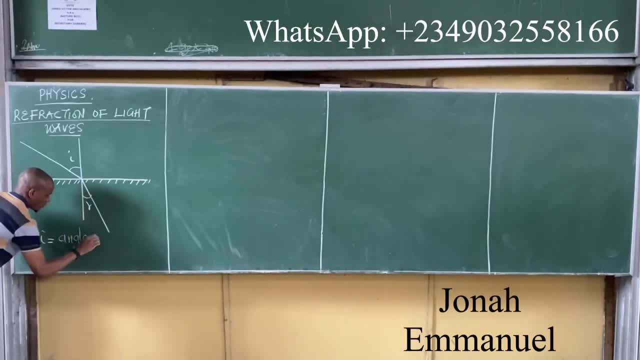 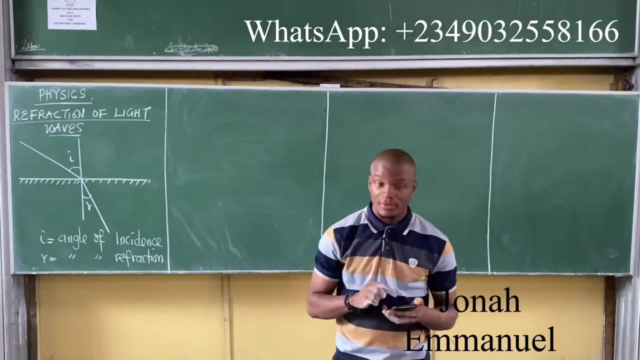 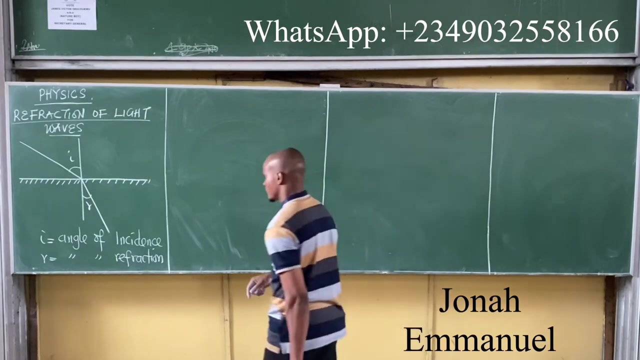 is equal to y, r is equal to the angle of refraction. all right, so here's the difference. so R in the first case was reflection, R in the second case is what refraction? all right, laws of refraction, laws of okay, hold on, hold on, hold on, look at me. 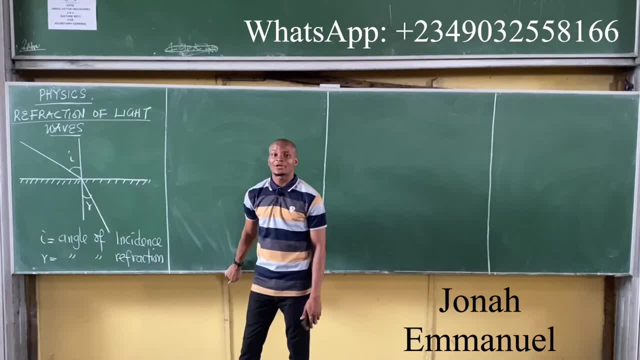 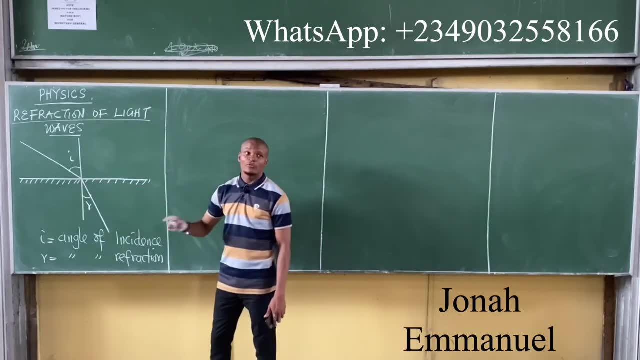 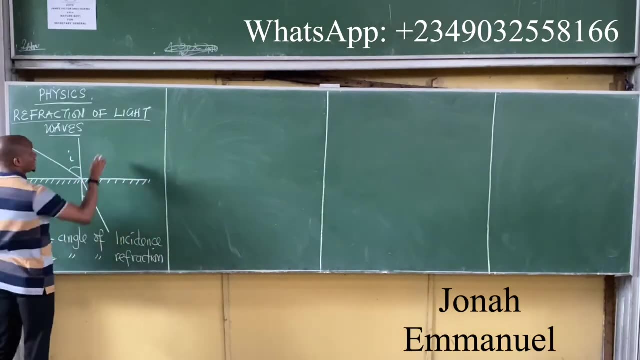 look at me now, see. i'm not different between reflection and refraction. For reflection, I was equal to I. For refraction, I is not equal to I. For refraction. two things exist: It's: either I is greater than I or I is less. 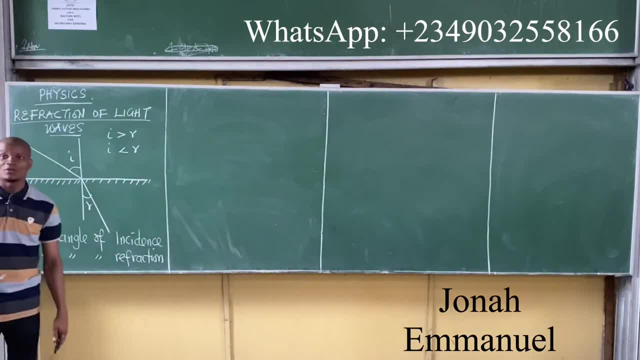 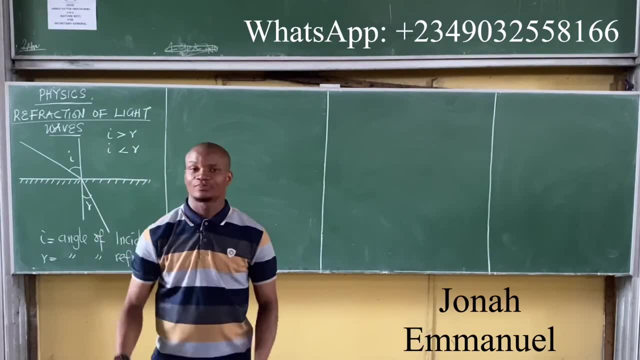 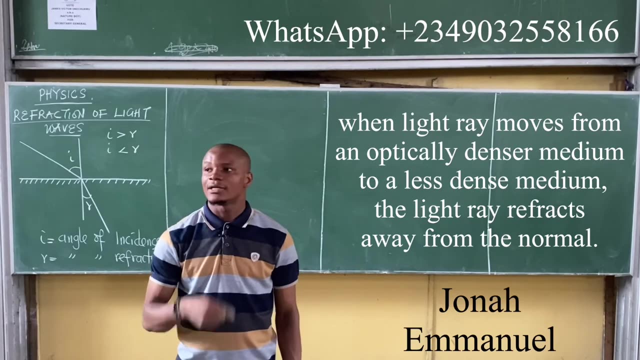 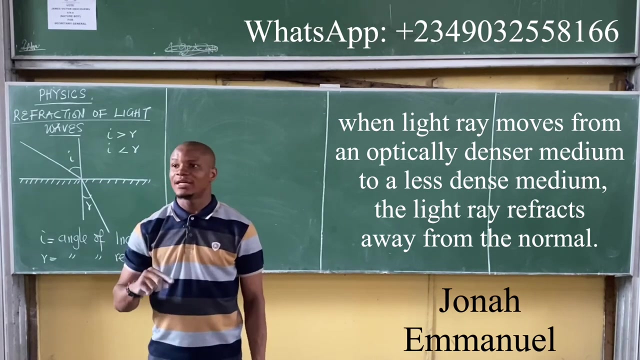 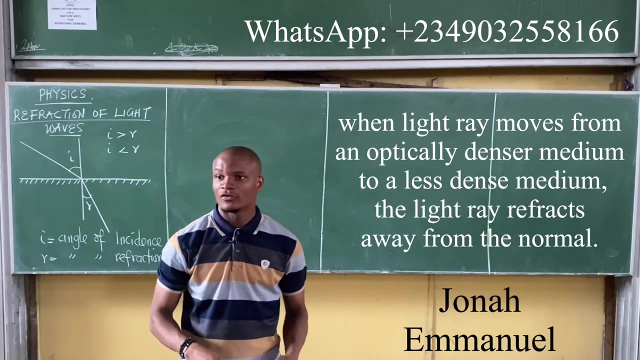 than I? When is I greater than I? In what case? Also, two: In what case is I less than I? Take that into note. When light ray moves from an optically denser medium. when light ray moves from an optically denser medium to a less dense medium, from an optically 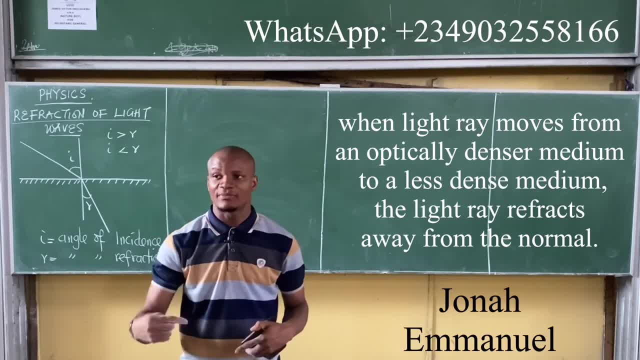 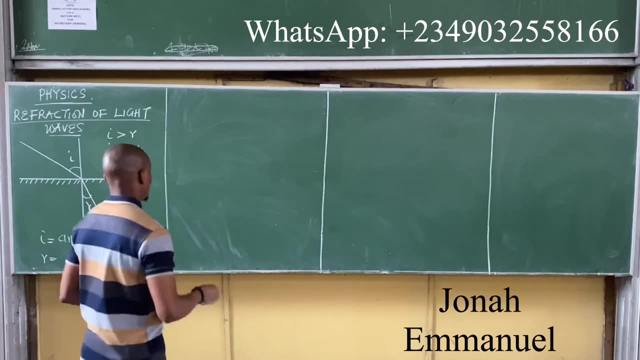 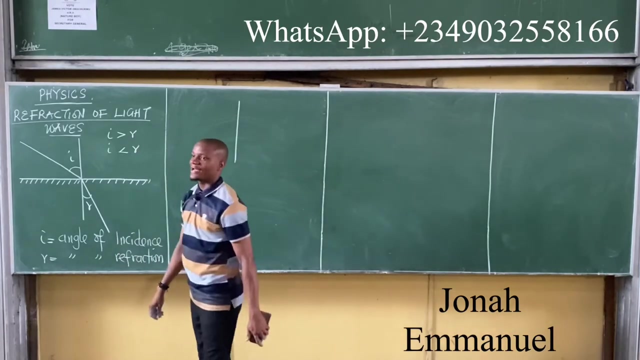 denser medium to a less dense medium. come back: The ray refracts away from the normal. The ray refracts away from the normal. Example Example: Let's use air and glass. Between air and glass which is more dense, which? 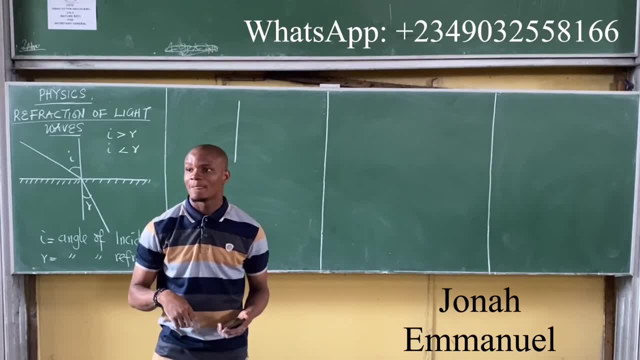 is less dense. Light and glass. Huh, Light and glass, Really, Please. Glass is denser. If you study optics and physics, you will see the word more dense. But more dense is not proper. all right, The word is what, Denser, Denser. But if you say 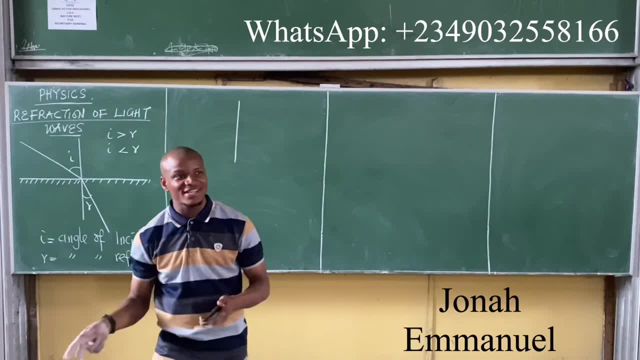 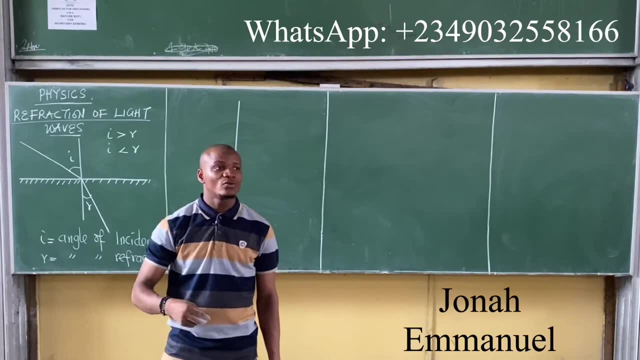 more dense, more dense, less dense, more dense, it's going to be denser. and you know, throw away. When it comes to listen, listen, listen. When it comes to density, what's density, What's density? 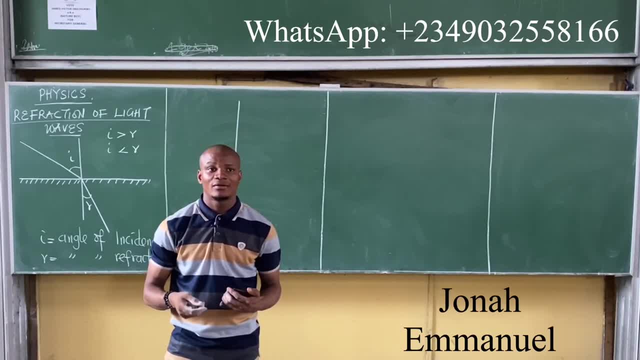 What's density? Decisively? whatever The ratio of light in mass per unit water, volume of light and object, the body, whatever. How do I know a body is denser? It's easy. It's easy If. 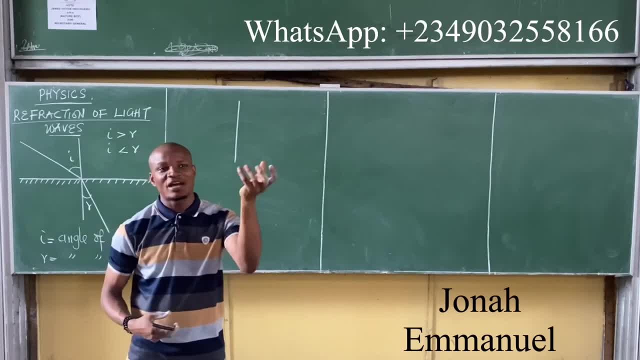 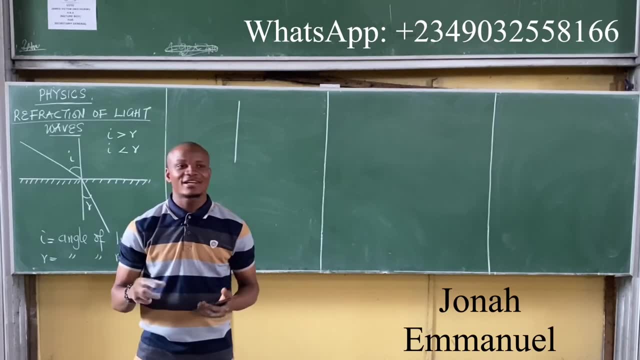 I have one hand like this of air and one hand of glass, which is heavier, right. So it's like a simple analogy for classifying density. Yeah, Yeah, So it's like a simple analogy for classifying density, Right. 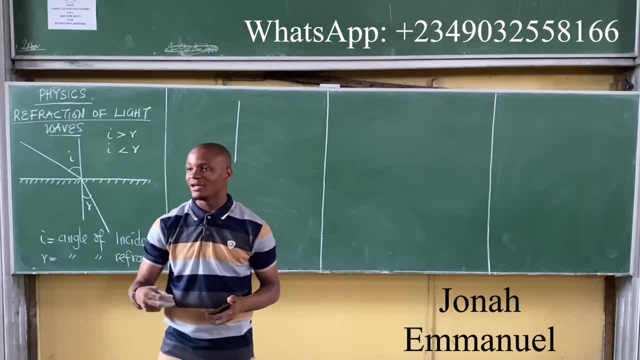 So it's like a simple analogy for classifying density, Right, Yeah, Yeah, Yeah Yeah. Usually, the heavier the object water, the more dense it is. Why? Because an object is heavy. Why? Because you have many particles. 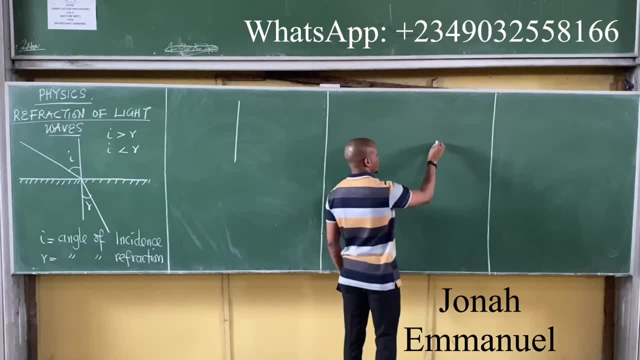 See something: When it comes to analyzing density, we are saying: in a particular volume, I have some mass in it. This density thing, In a particular volume, I have some mass in it. Right, The concept is this: now, The more mass like this, now, the more masses I have in this volume, the more dense it is. 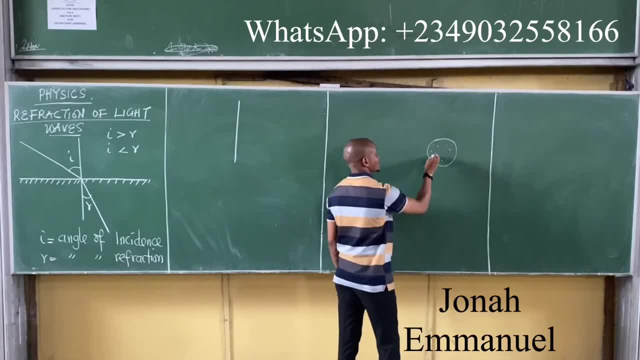 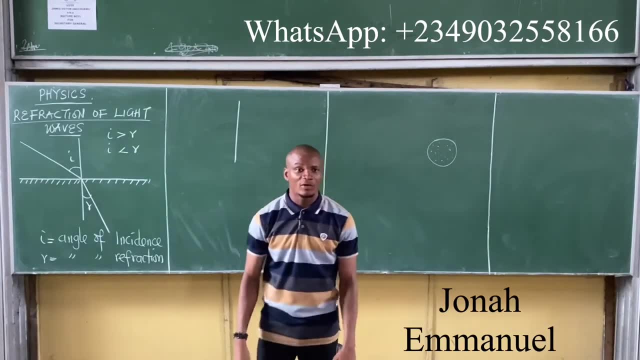 And that's how you see that Usually heavier objects tends to go there more dense than what Lighter objects, Just like the case there. What does it mean? It means that what Glass is what More dense than what Than air. 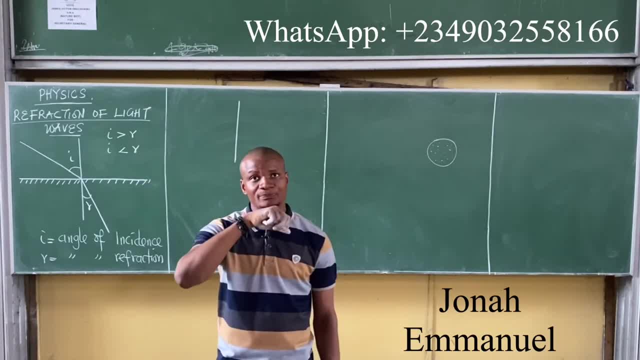 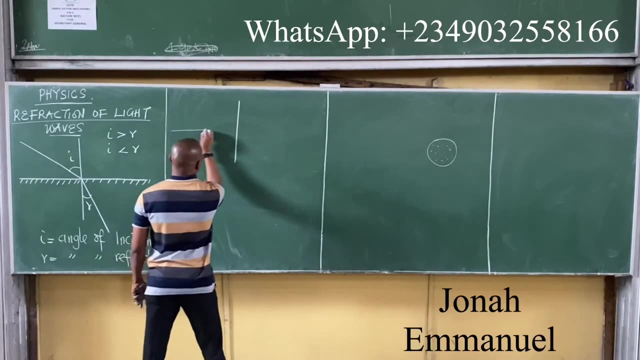 Now we just said something there. We said if light ray is moving from what It's more dense than what A less dense medium, What happens to it? It refracts what there Away from the normals. Look at that. So I will use two things there. I will use the more dense. So from a denser medium, let's say glass, to a less dense medium. 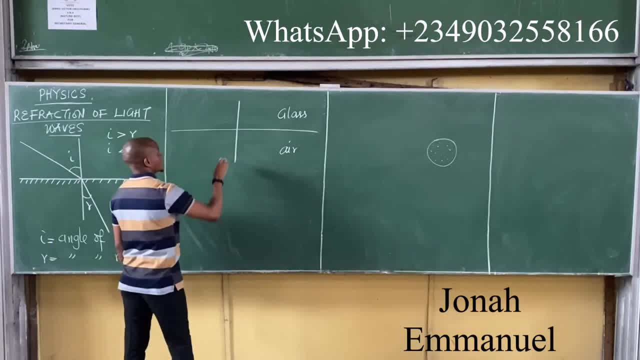 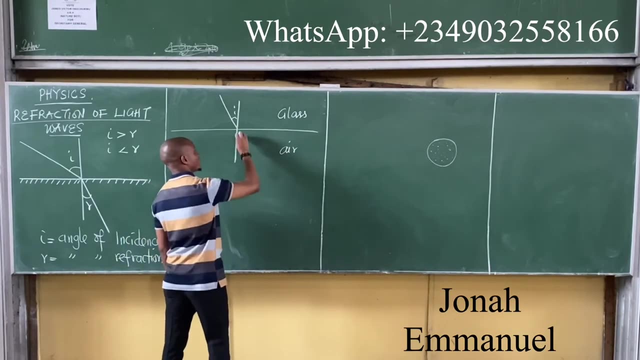 Let's say, for instance: Alright, So here's my normal, This one goes this way. Alright, So here's my angle of incidence In this case. we said it reflects light. It refracts not close to the normal, but there, away from the normal. 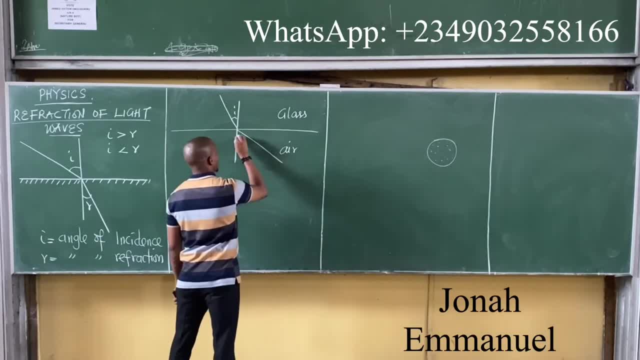 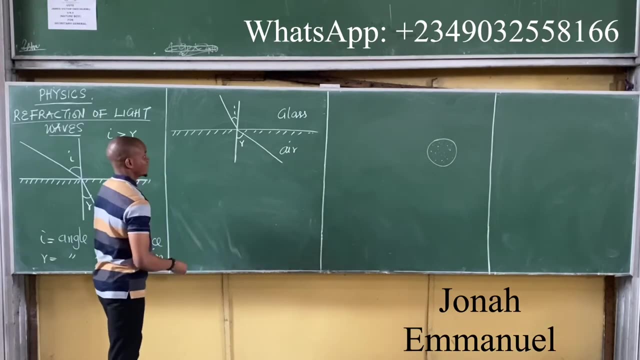 So it's doing something like this, Something of this nature? It's going away from the normal, Away from the normal, Alright, So from here it's going, as I said, shooting outside this line. So it's going away from the normal. 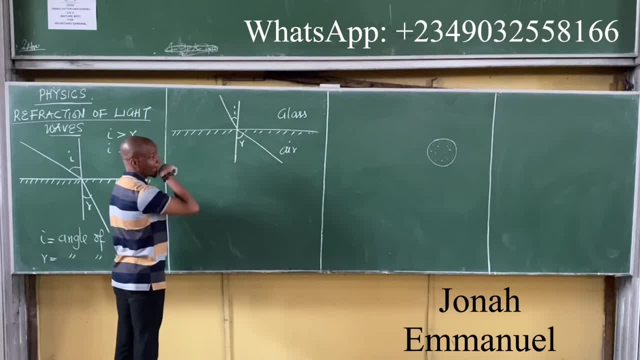 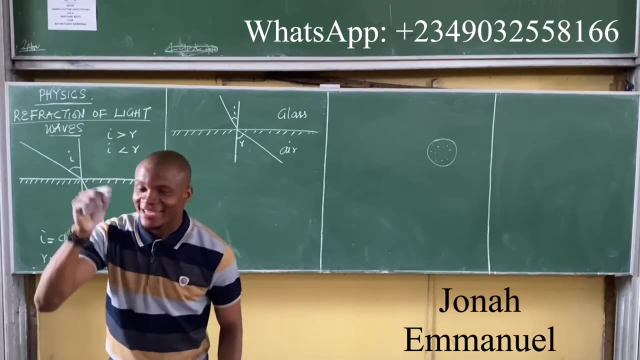 In this case here, between I and I, which is greater? I'm not In this case now, between I and I. which one is greater? I, I, I. What are you saying Between I and I? I and I. 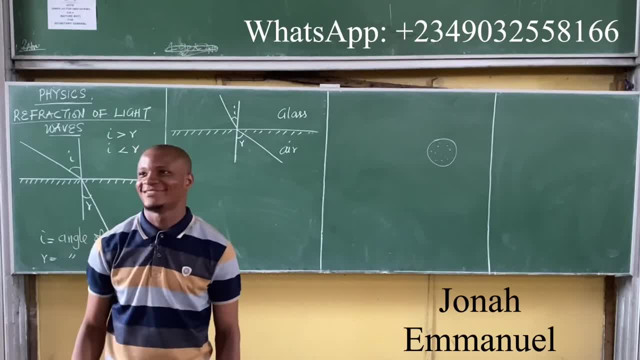 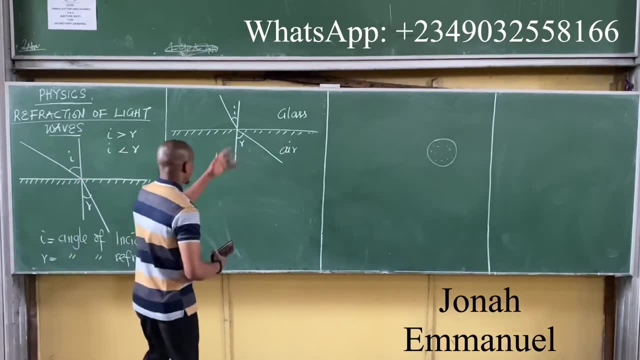 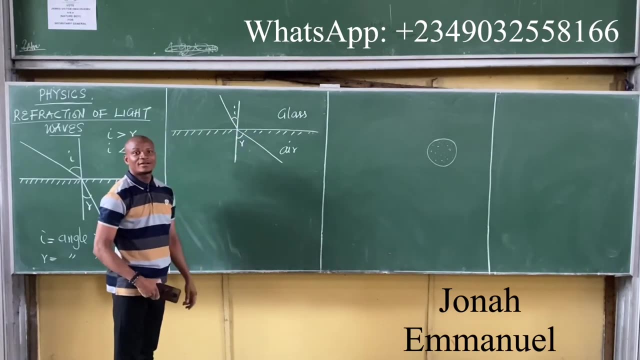 Not I. What are you saying Between I and I, please? Which one is greater? I Look at what you have here, See, I See I, I is on here. Which one is greater? I? I Wait, Wait. 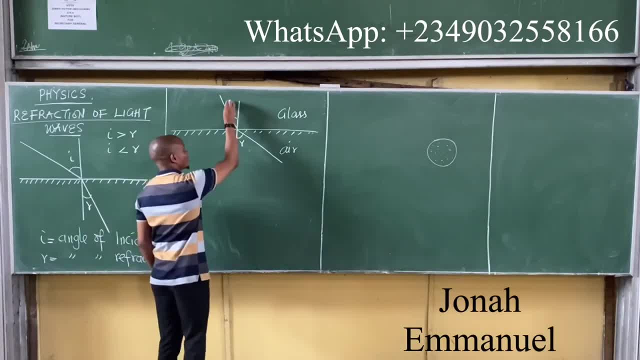 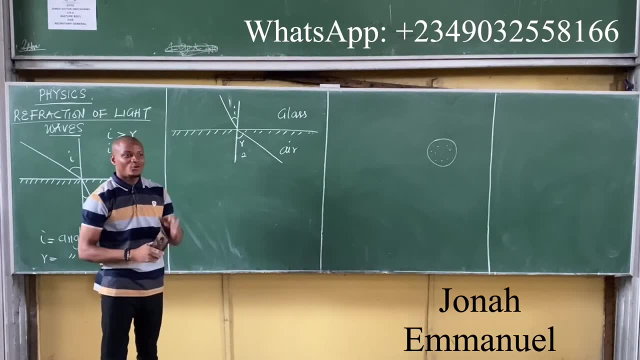 Hold on, Hold on, Hold on, Don't worry, Leave I and I See one. See two, Between one and two, which is greater Two, Hold on. Let me show you what I'm saying. See, See one here. 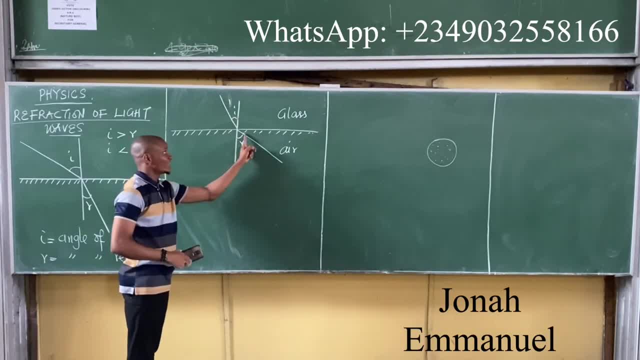 See the angle of one. See the angle here. Two is this, one here, Between one here is I and two, which is greater? Two, Two is greater now. So what does it mean? It means that one there, one is what? 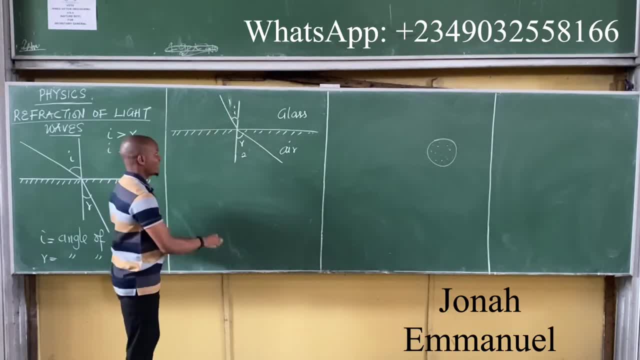 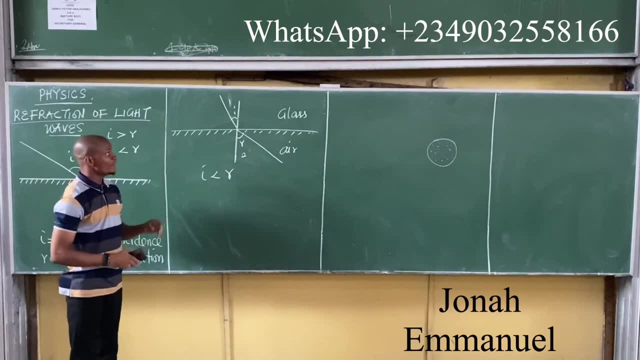 Less than what Two. So what does it mean here? It means I is one there less than what I. So here's the condition: A wave moves, or a light wave moves from a dense sand field of the world a less dense. 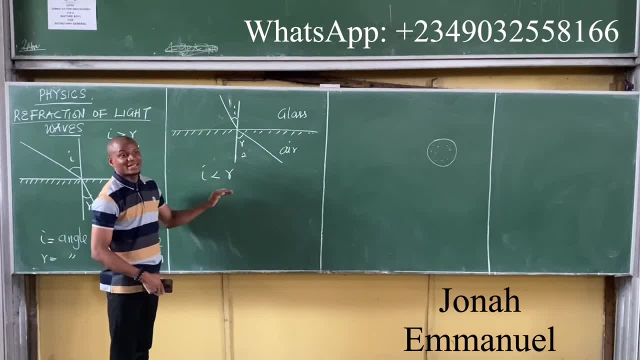 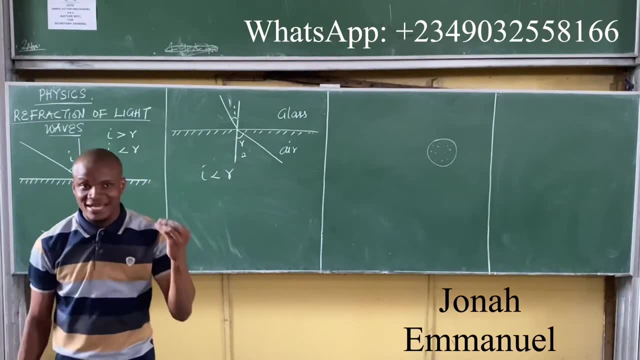 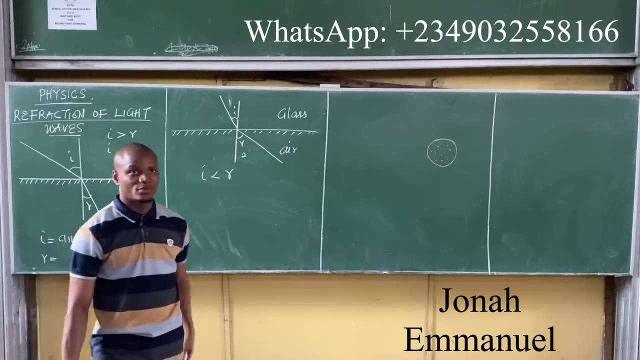 in the water there than the world? is the world less than the angle of refraction? That's it. It moves from a denser to a less dense. I becomes less than I. That is identity. Yes, What's the question? 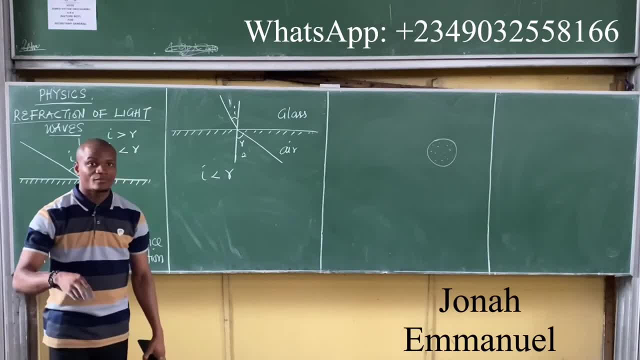 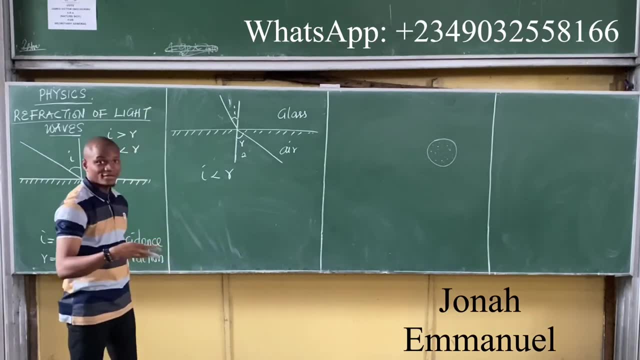 So if you're going like this, you're not going to mix and mix and mix and mix. Look at me first, See what you're saying. You're going like this: Right, What's like this? Each path, Please, Please. I'm not moving this way. 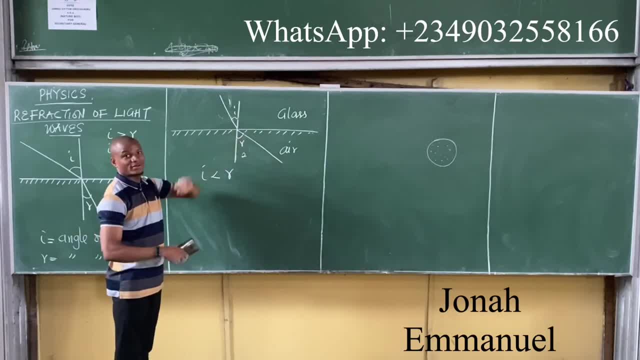 Just like this. So it's just this hand here and then this hand here. Can you tell me which side is light? Which side is light? Which side is light? This side is light, This side is light. I think this one is closer. 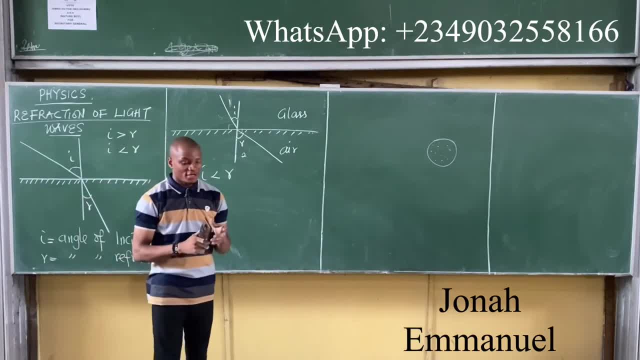 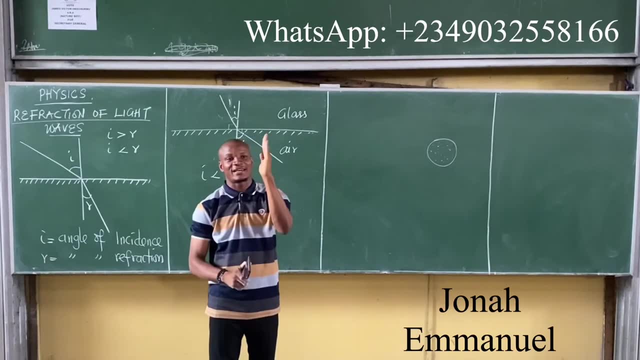 to light If it's closer to light, if it's closer to see. see an arm here. If my phone is closer to look at this now, Look at this now. So let's take this as light here In this case. now. 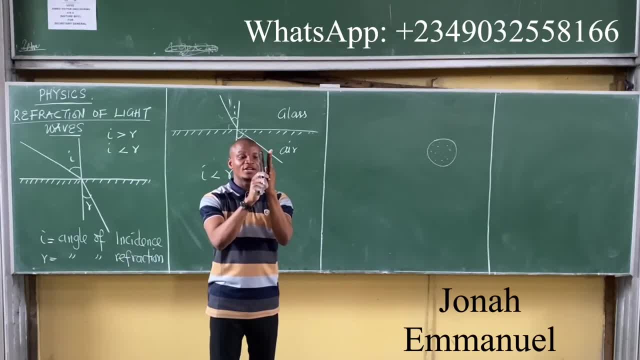 my phone is closer to this, one like this: This case one, Case two: My phone is farther from here. Which is greater? Huh, First, or the second case? Huh, Talk, and let me know which one is greater. You don't know. 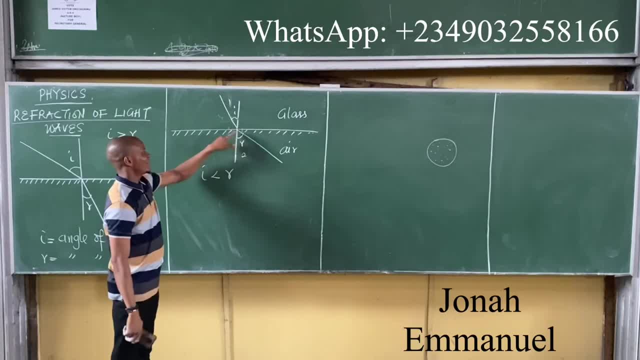 I don't know how you imagine. Listen, Listen, Listen. Are you doing like this way? Is that what you're doing? Don't leave the light here. We're not considering light in this case. You're only looking at this arm. 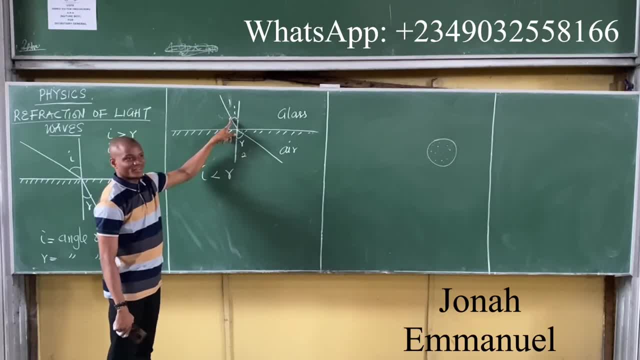 here. It's not even moving. It's the way it is. It's not moving. Stop moving it. It's not moving, Stop moving it. I think what you're doing is this: You're looking at it and it's going this way. 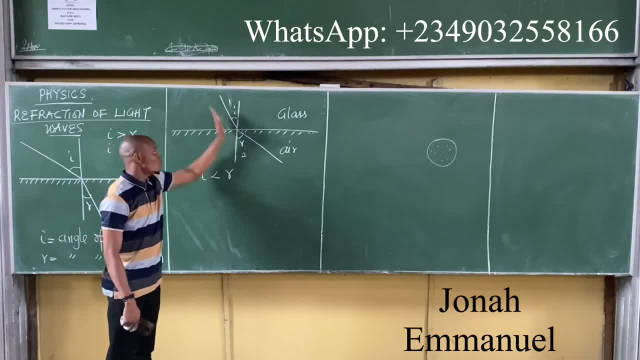 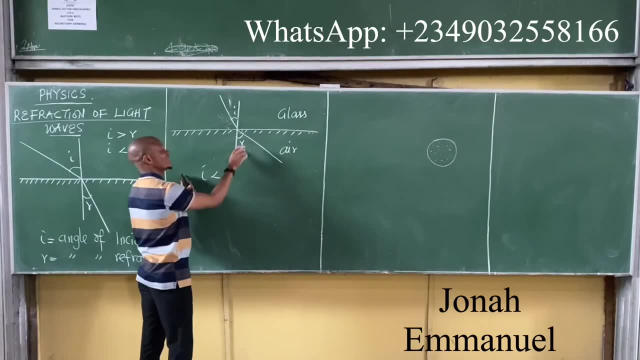 So it has the bigger distance. That's not it. This is the way it is here. In this case now, this one is closer to here. In this case, this one is far from here. Obviously, the farther one will have the bigger arm in the water. 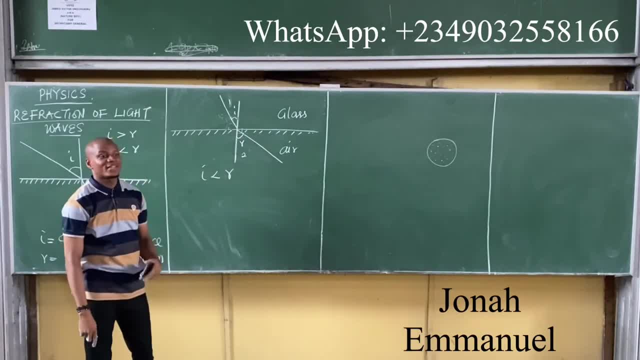 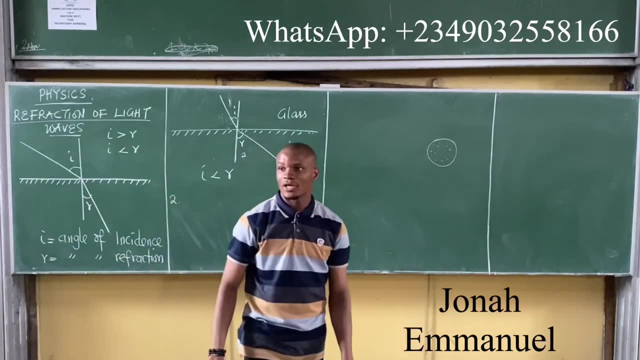 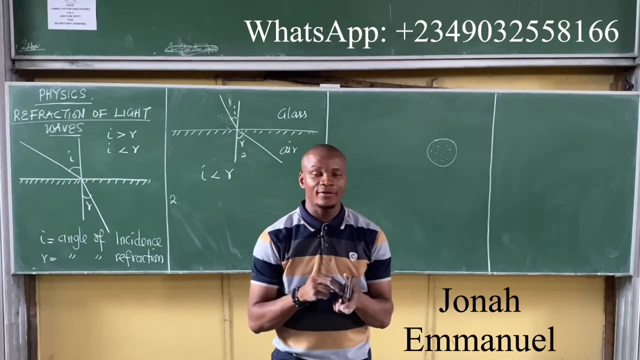 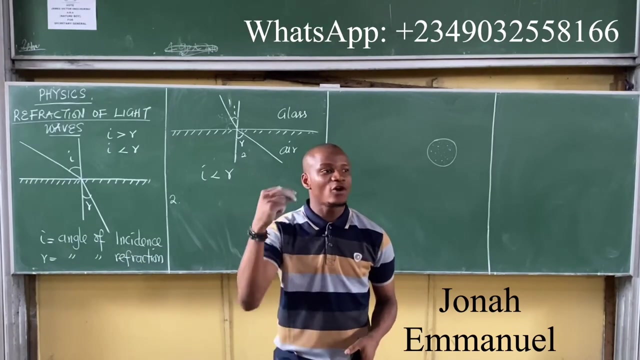 The closer one. That's what you're saying. So I become less than I. Case 2,, please. Case 2.. Case 2. If light ray. Case 2. If light ray moves from an optically less than medium. 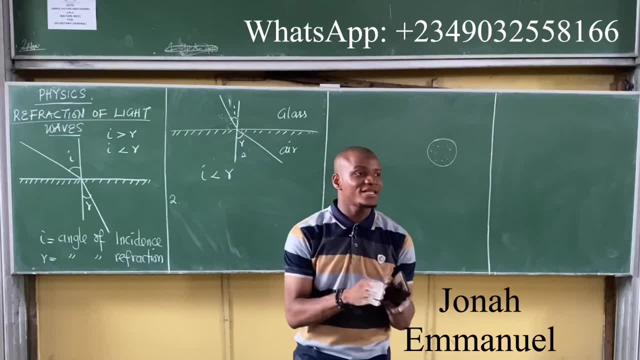 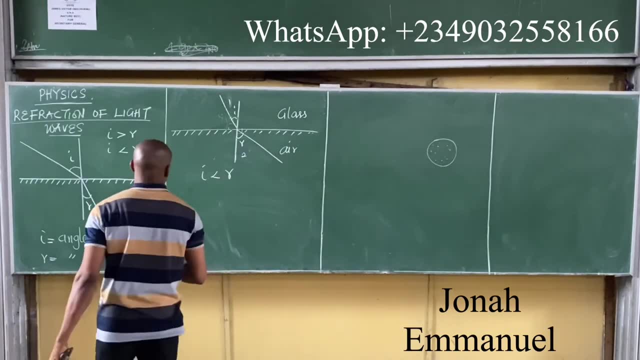 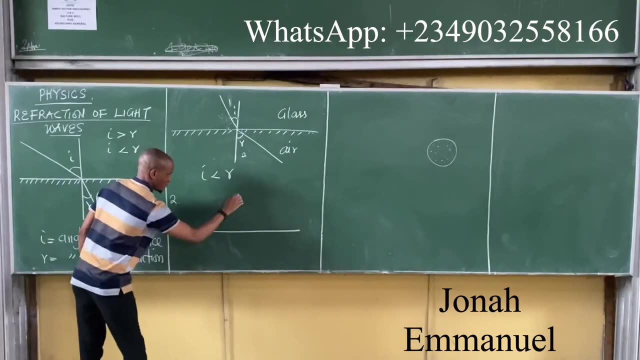 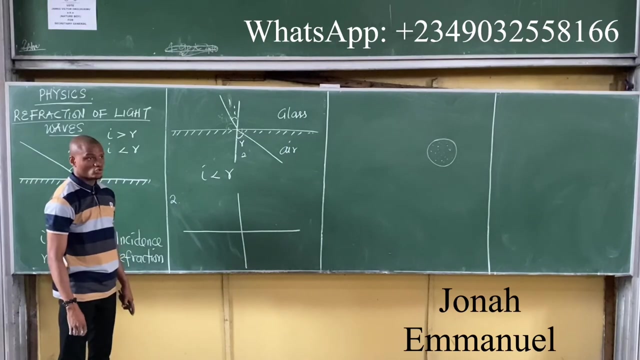 if light ray moves from an optically less than medium to a denser medium. if light ray moves from an optically less than medium to a denser medium comma, the ray will refract. closer to the normal comma, the ray will refract. 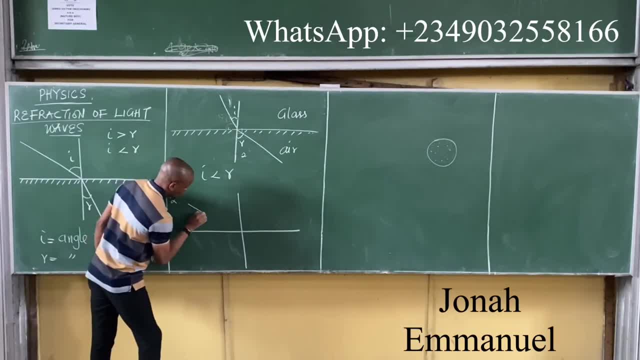 closer to the normal comma, the ray will refract closer to the normal. The ray will refract closer to the normal. Now, look at this, Look at this. See this arm here, In this case, now, the arm that will go over there, close to my normal. 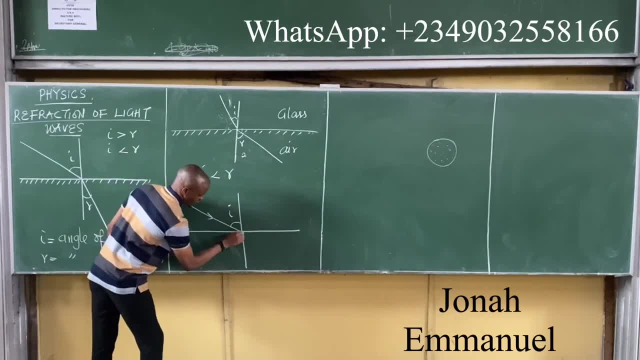 Now, that's the vertical line, so it will look like this, something of this nature: What do you attempt now? In this case? now it's refracting close to this number, In this case, obviously, what comes here? now We're taking this one as well. let's say air in this case. 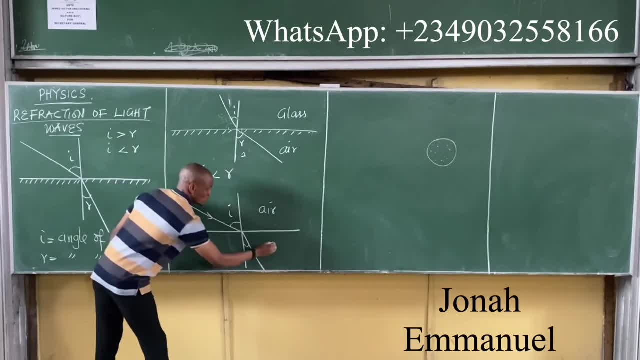 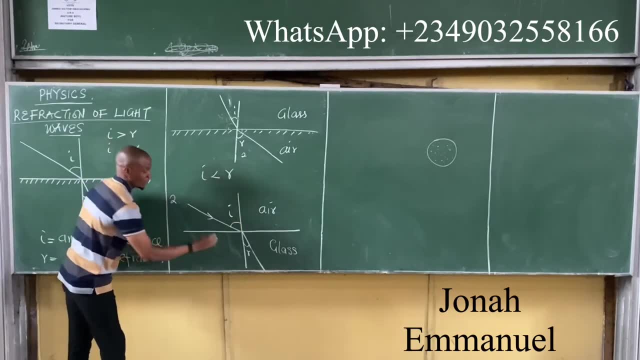 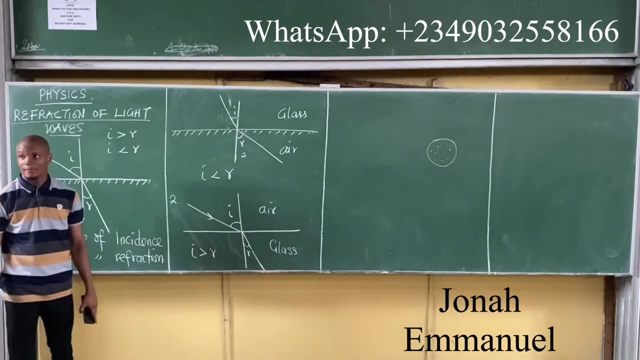 So, from air in less dense medium to, let's say, glass in more dense medium, what comes here? now You can see that air is greater than water air. so this case now, air is greater than air. That's it. Mind you, mind you, mind you. I can express it in two forms. 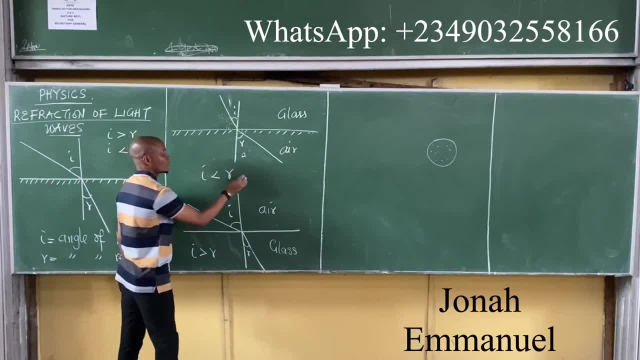 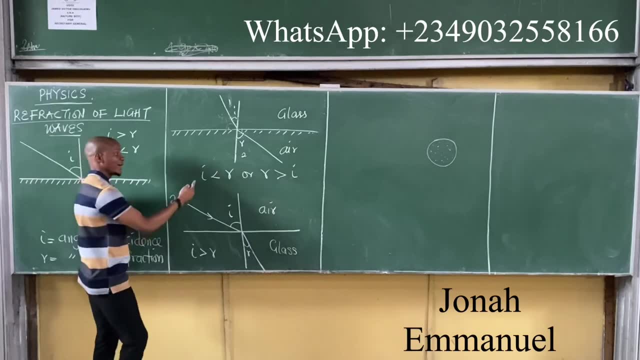 It's either. you see, air is less than air or water. air is not water greater than water. air, It's the same thing That air is less than air or air greater than water. It's greater than air. In this case, air is greater than air or water. air is what. 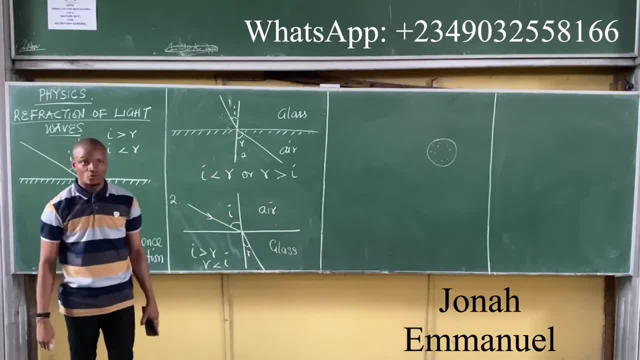 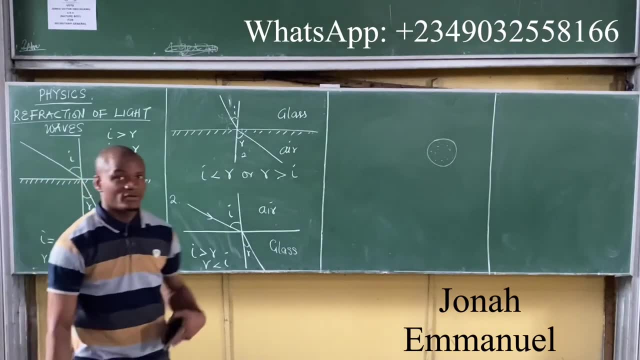 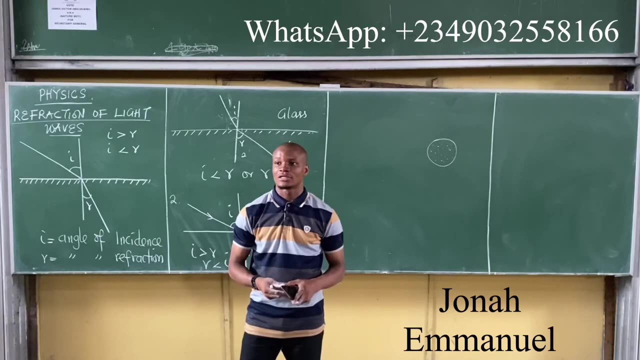 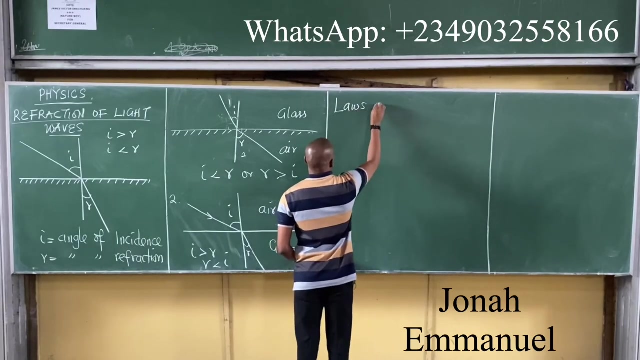 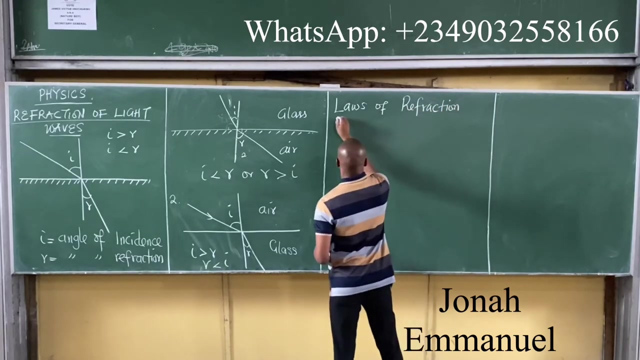 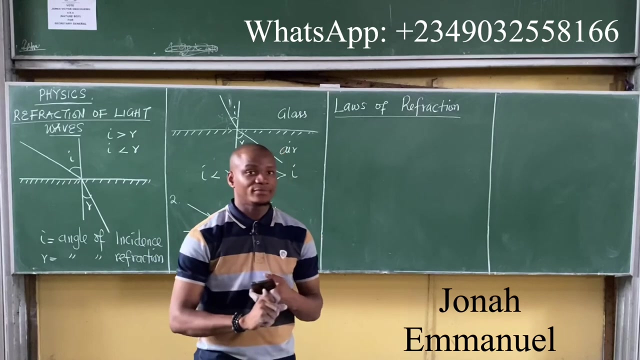 Less than air, whichever one it is. So we are seeing something very simple. What's that? Air cannot be equal to air in refraction, So it's the same, Alright. Law of refraction. Law of refraction Number one. 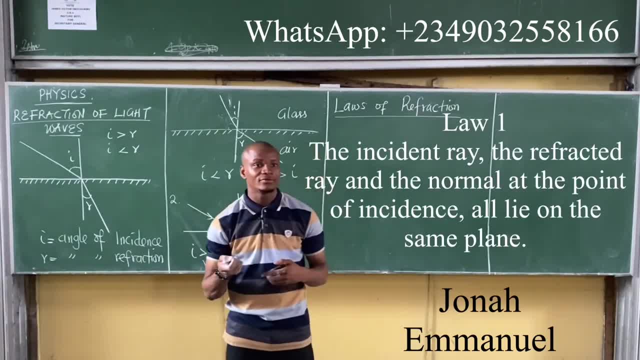 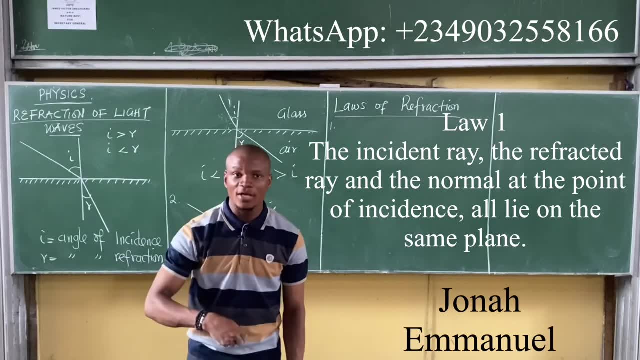 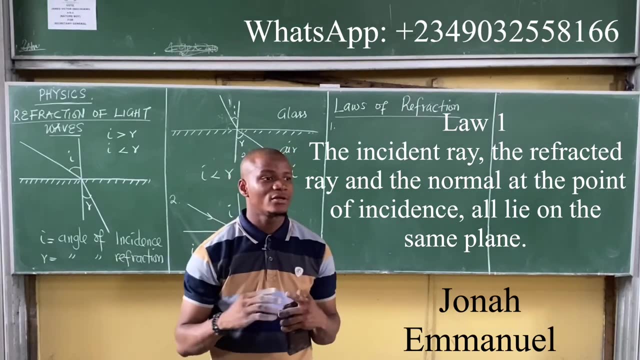 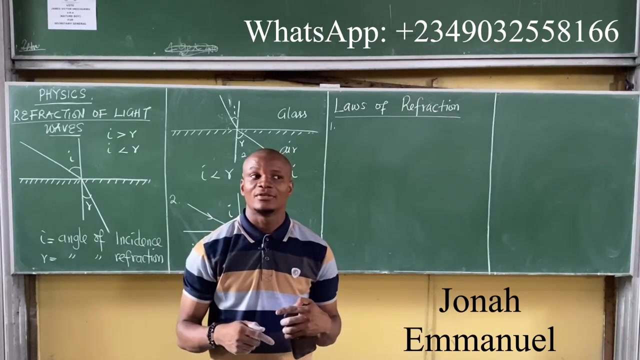 The incident rate, the refracted rate and the normal at the point of incidence and the normal at the point of incidence all lie on the same plane. So we are seeing that, if you observe, the first law of reflection and the first law of refraction are like the same thing. 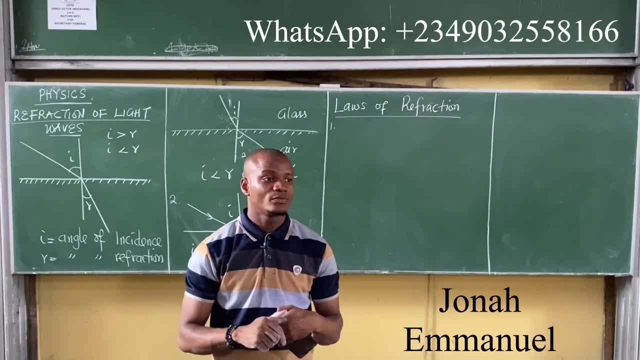 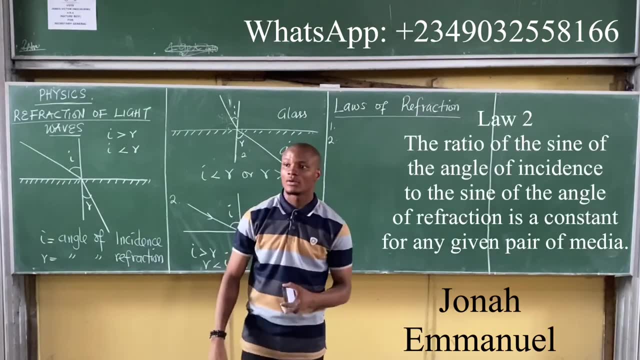 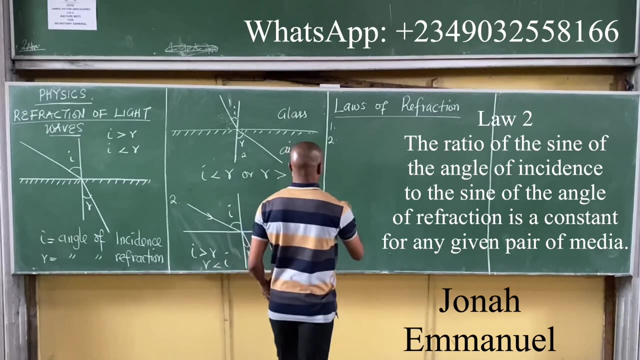 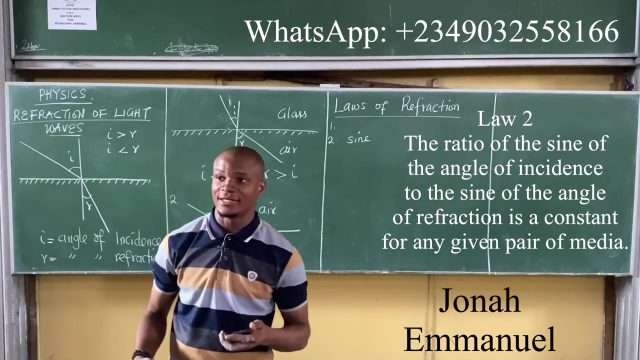 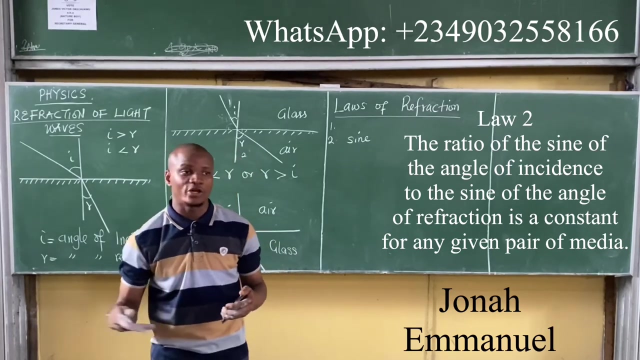 Yeah, Number two. Number two: The ratio, the ratio of the sign, the ratio of this way, the sign of the angle of incidence to the sign, of the angle of refraction to the sign, the same sign of the angle of refraction. 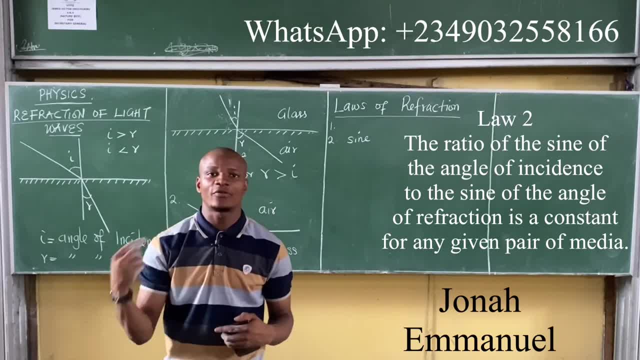 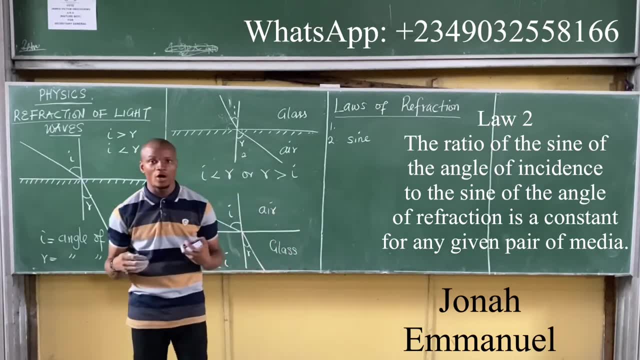 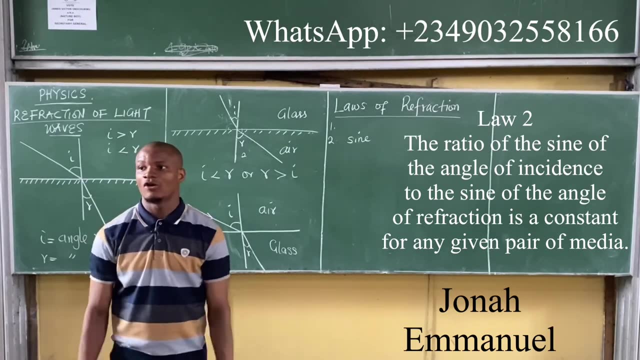 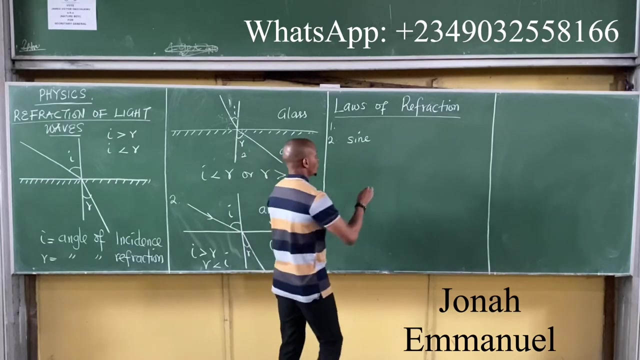 the same sign of the angle of refraction is a constant for a given pair of media. It's a constant for a given pair of media. This law- let me proceed. This law is also called Snell's law. Snell's law. 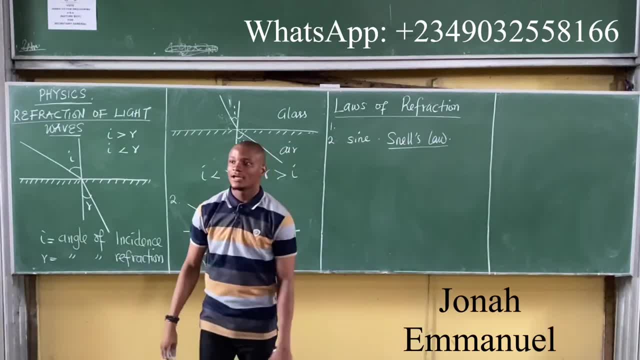 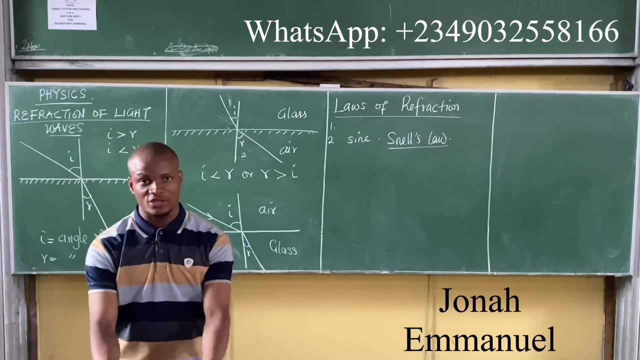 This law is also called Snell's law. So what's Snell's law? Snell's law is also known as the second law of refraction. It states that the sign of the angle of incidence to the sign of the angle of refraction is. 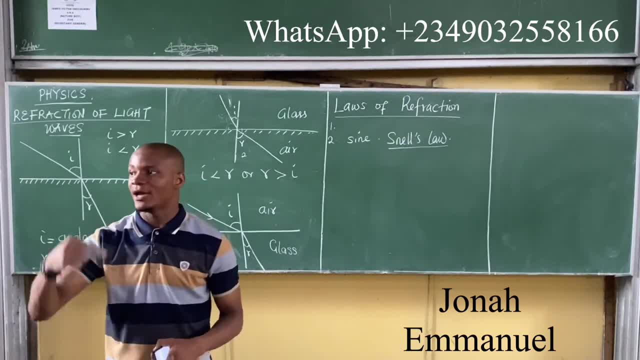 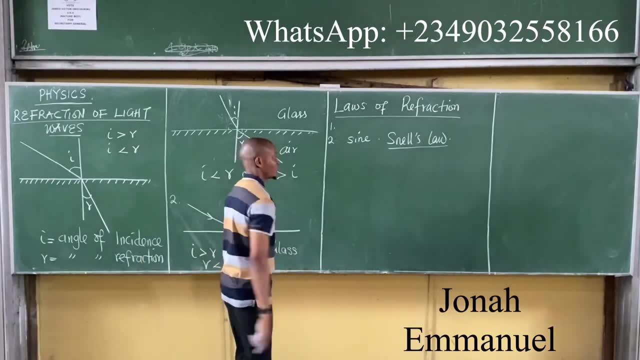 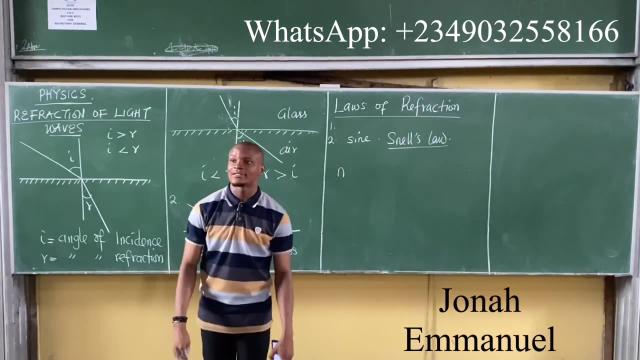 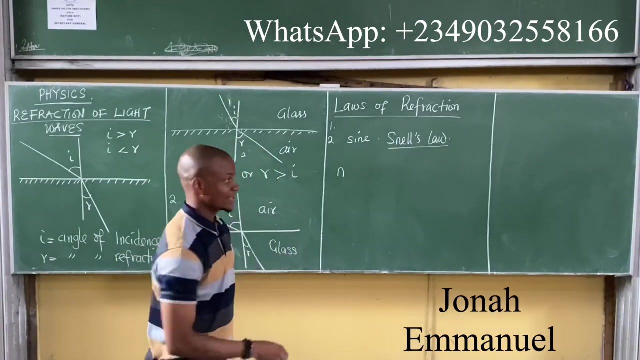 a constant for any given pair of media. That's all, This constant. who stopped This constant is right. This constant is represented by n. This constant is represented by n And it's known as the refractive index By n. 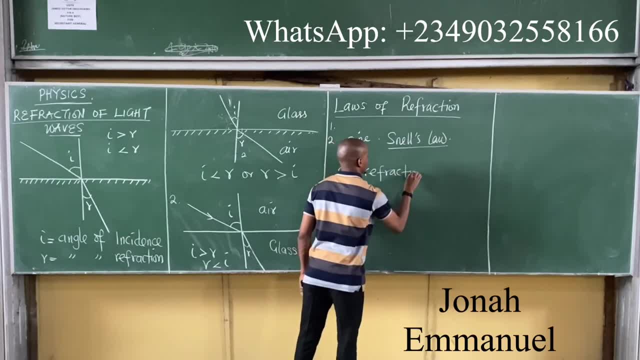 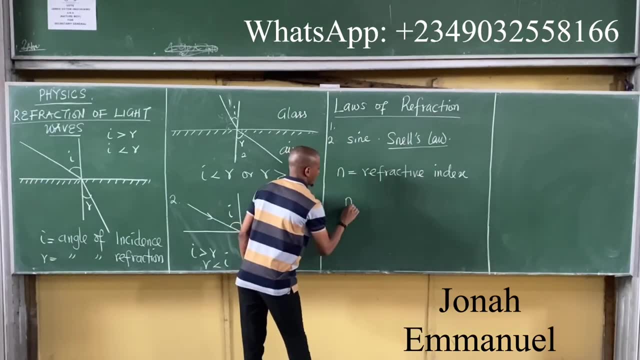 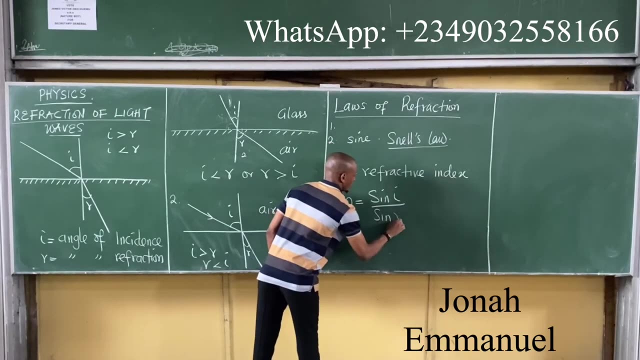 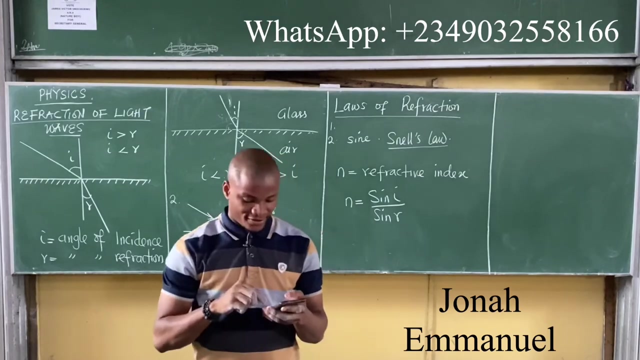 And it's known as the refractive index. By seeing that the refractive index n is equal to sign of the angle of incidence, The refractive index is equal to sign of the angle of refraction, Refraction, Refraction. 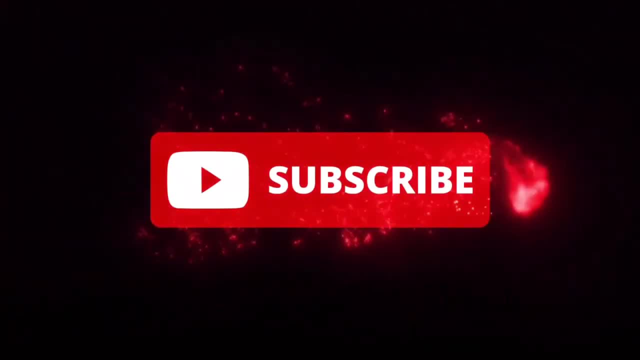 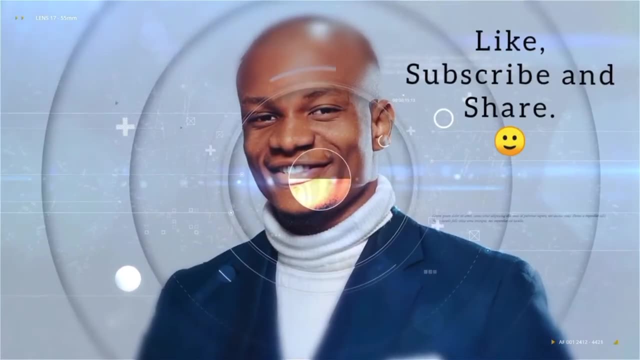 Dawel Lamb wwwthriveamjcom.